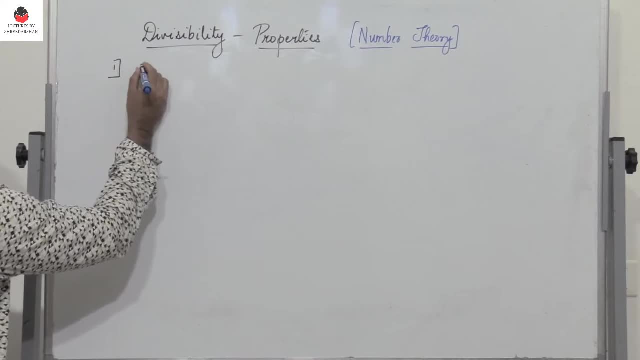 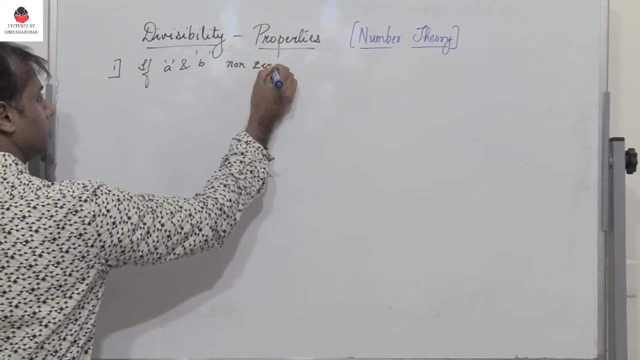 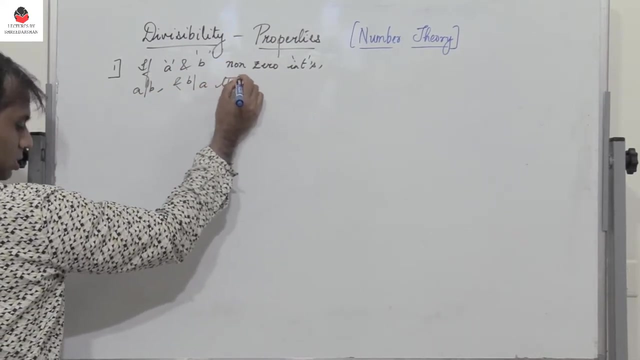 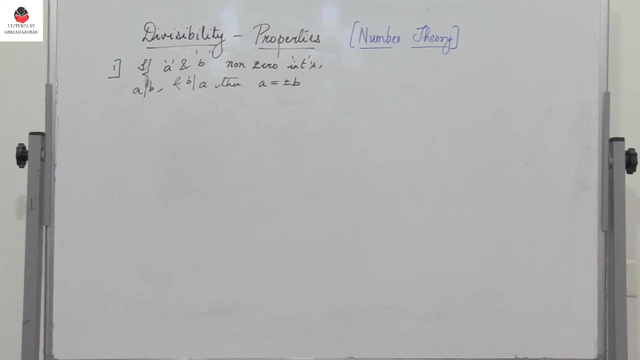 of divisibility. The first property: if A and B are non-zero integers, such that A divides B and B divides A, then we can say that A is equal to plus or minus B. So here A and B are non-zero integers and A divides B and B divides A. So how do we prove this? So let us see the proof. 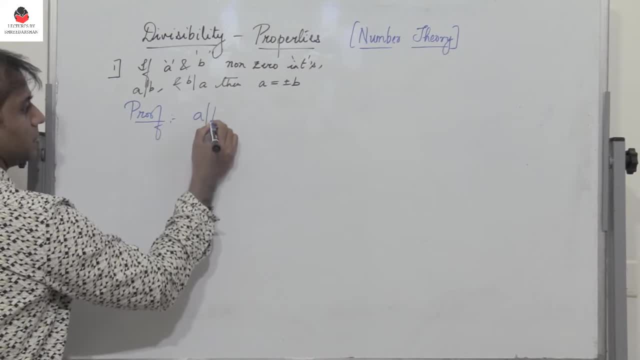 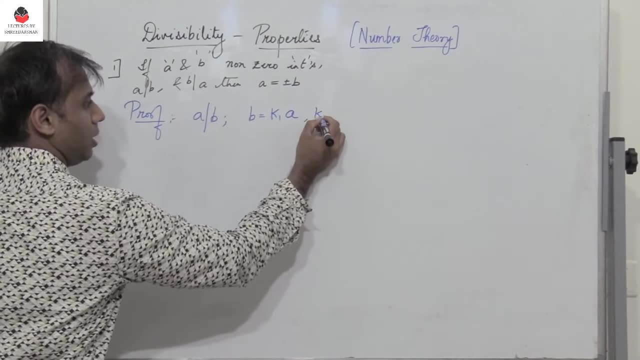 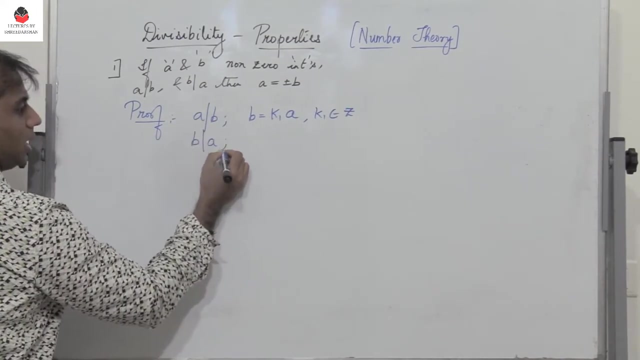 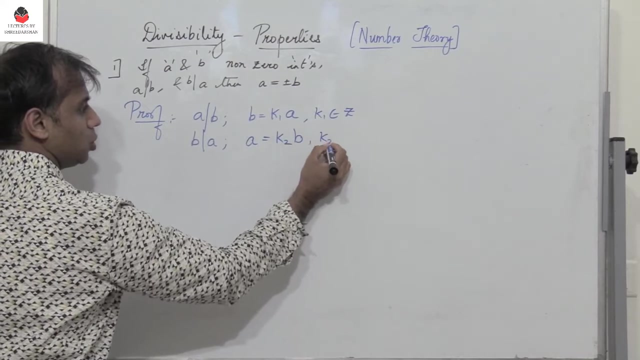 So since A divides B, so A divides B, which means B can be written as some constant K1 into A Right. So where K1 belongs to the set of integers, Now, similarly, since B divides A, I can write A equal to another value, K2- into B, where K2 belongs to the set of integers Z. Now I call this as 1.. 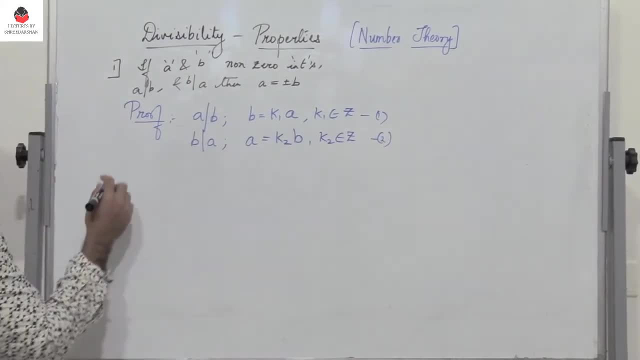 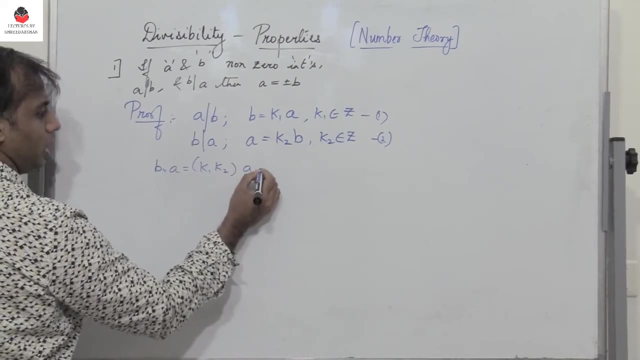 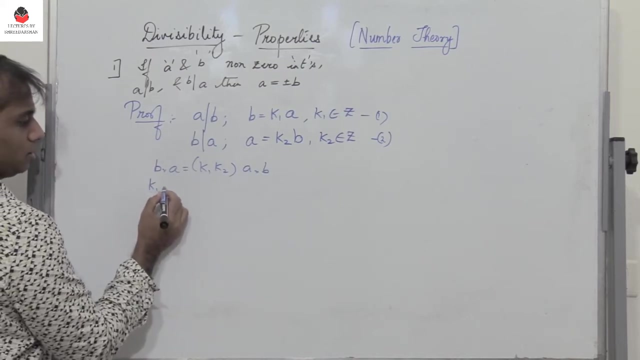 And this is 2.. Now multiply 1 and 2. So you have B into A equals K1 into K2, into A into B. Now, when is B into A equal to A into B? So this happens when K1 is equal to K2 is equal to 1. 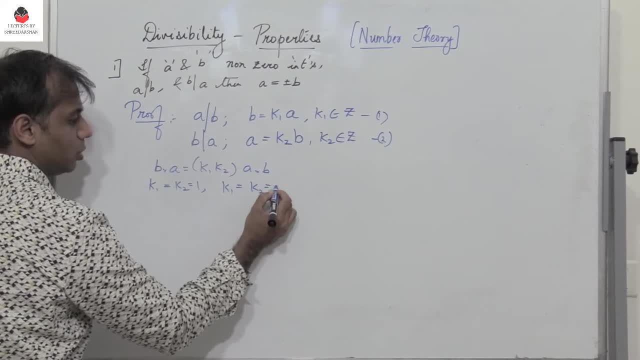 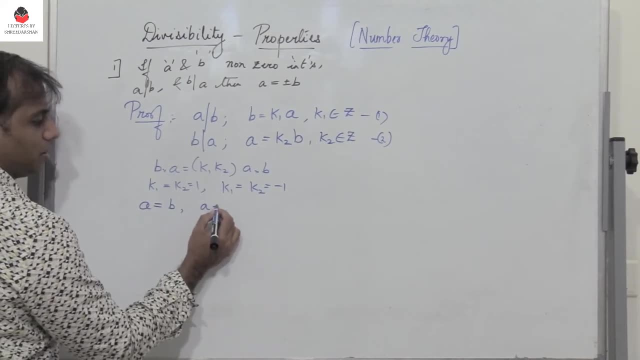 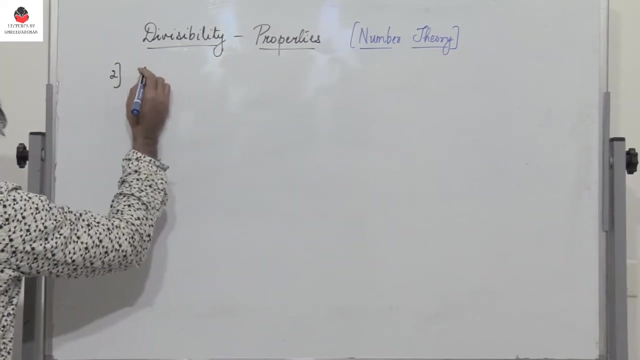 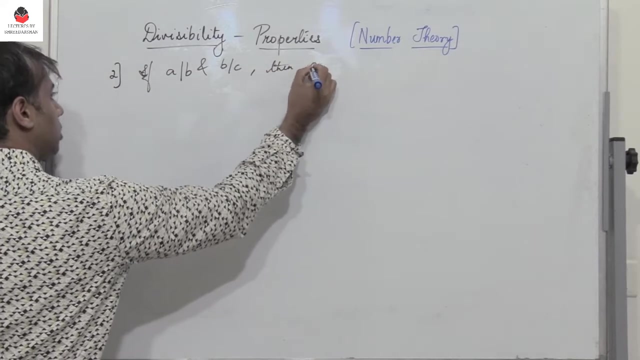 or K1 is equal to K2 is equal to minus 1.. Or we can say that A is equal to B or A can be equal to minus B. So therefore we say that A is equal to plus or minus B, The second property. if A divides B and B divides C, then we conclude that A divides C. 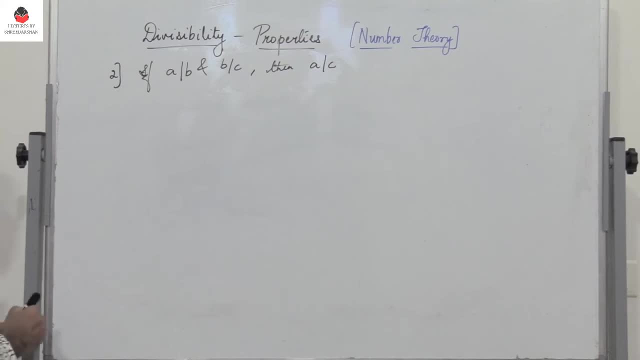 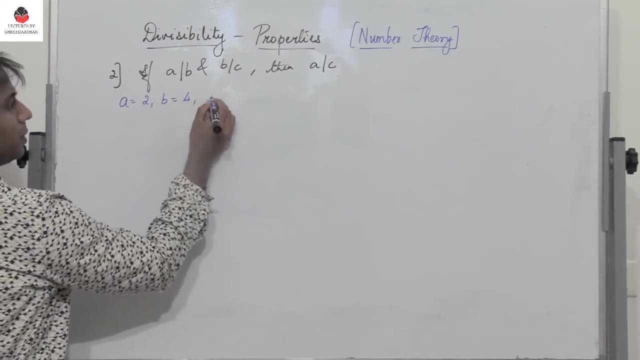 Now how do we prove this? So let us first take an example. Now, if A is equal to 2 and B is equal to 4, and then if I have C, then I can write: A is equal to 2 and B is equal to 4.. So this is a. 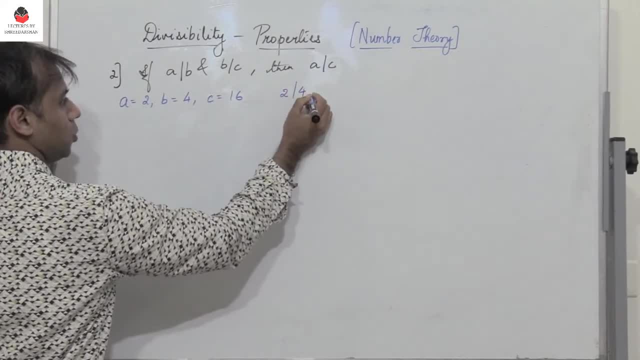 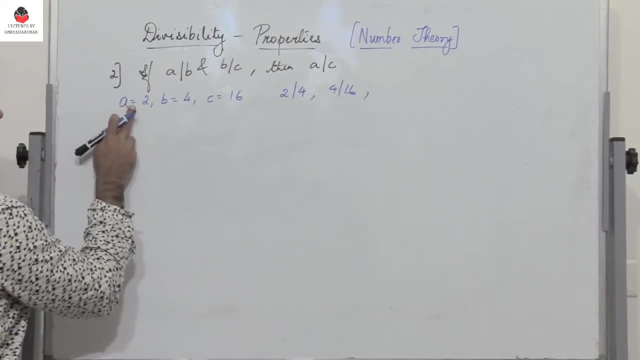 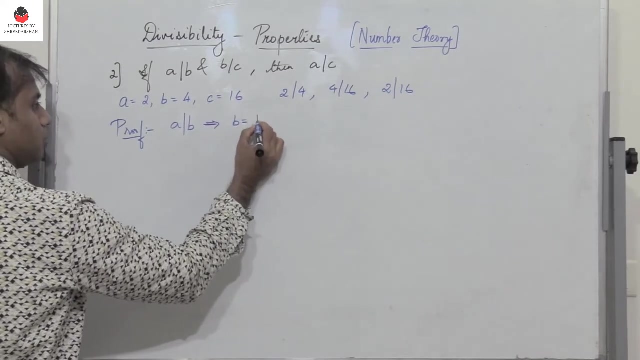 16.. We know that 2 divides 4 and here we have 4 divides 16, which is B divides 16, and also A divides 16.. So 2 divides 16.. A divides B, which implies that B is equal to K1, into A. Call this: 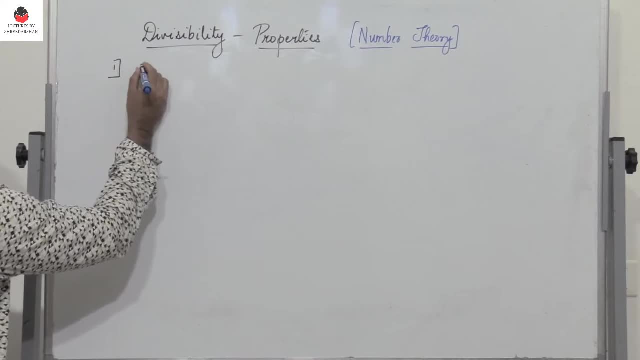 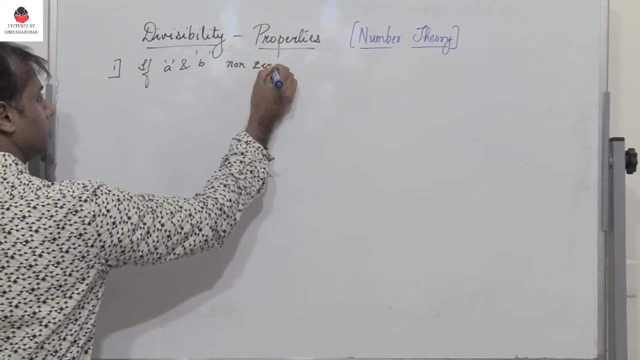 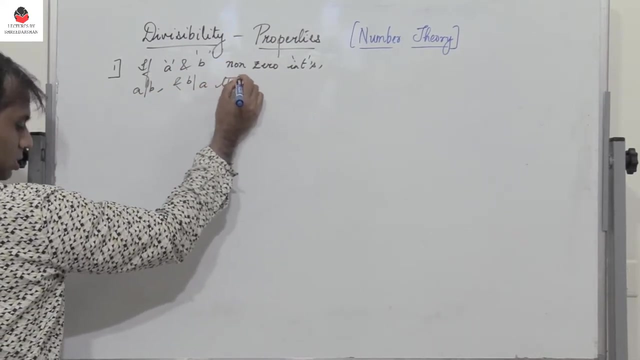 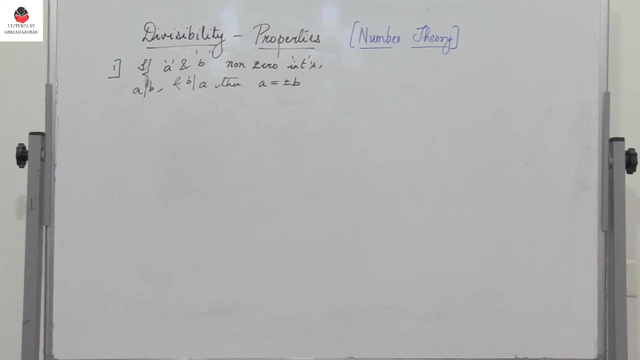 of divisibility. The first property: if A and B are non-zero integers, such that A divides B and B divides A, then we can say that A is equal to plus or minus B. So here A and B are non-zero integers and A divides B and B divides A. So how do we prove this? So let us see the proof. 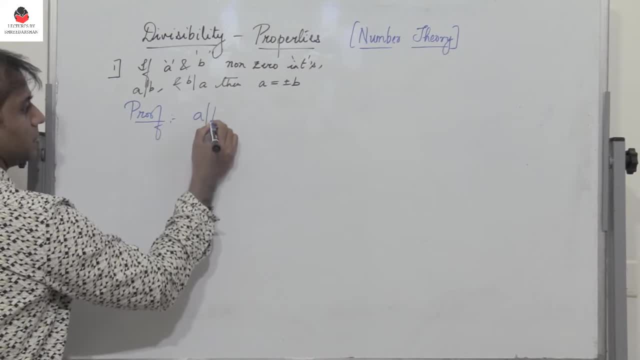 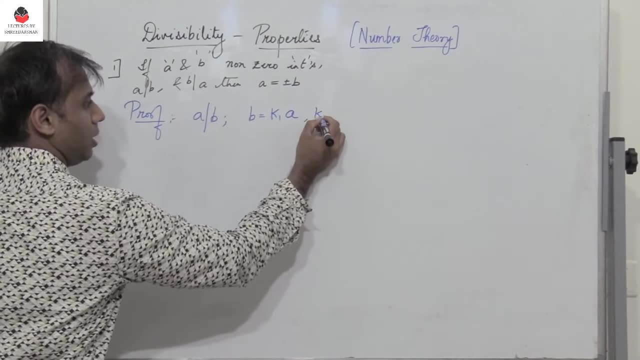 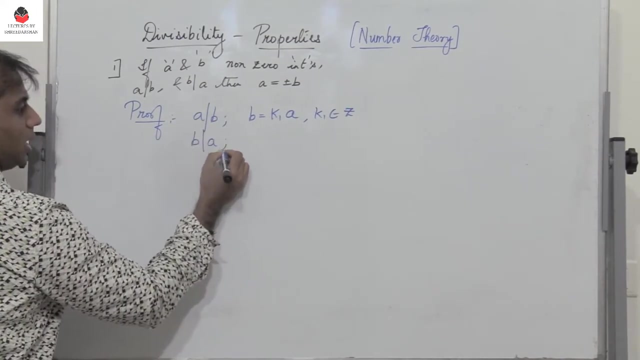 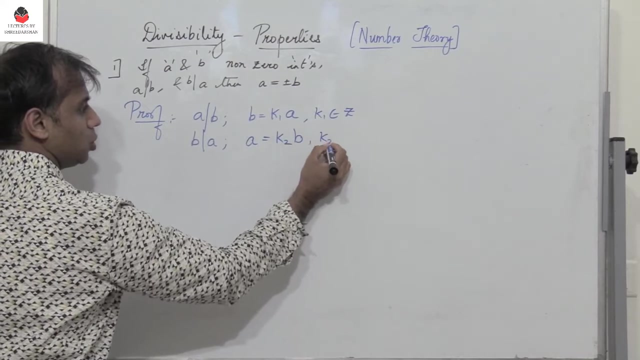 So since A divides B, so A divides B, which means B can be written as some constant K1 into A Right. So where K1 belongs to the set of integers, Now, similarly, since B divides A, I can write A equal to another value, K2- into B, where K2 belongs to the set of integers Z. Now I call this as 1.. 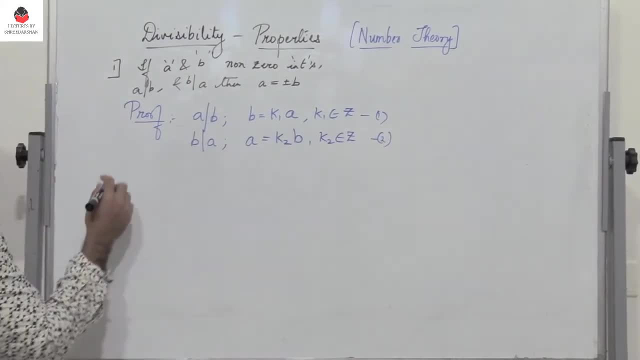 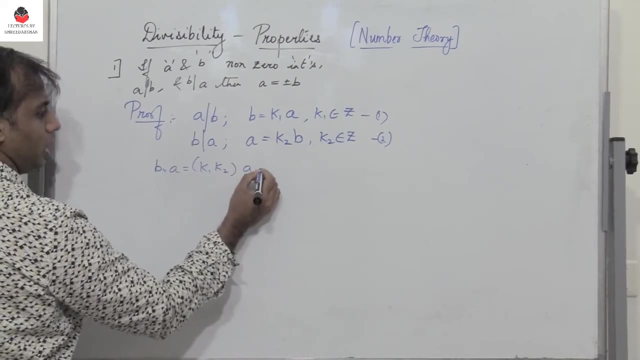 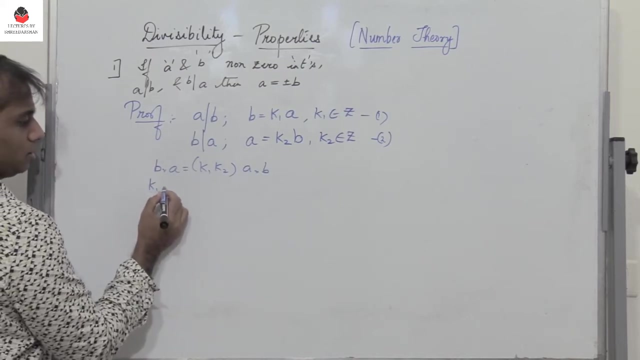 And this is 2.. Now multiply 1 and 2. So you have B into A equals K1 into K2, into A into B. Now, when is B into A equal to A into B? So this happens when K1 is equal to K2 is equal to 1. 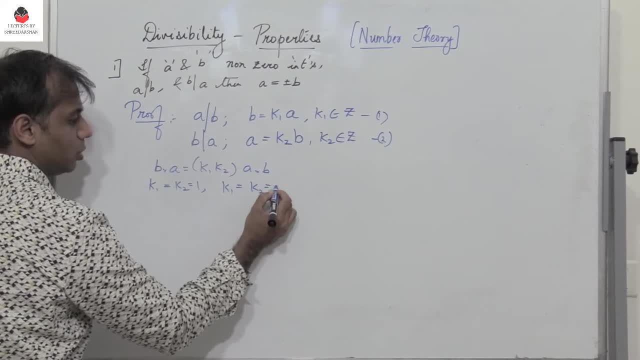 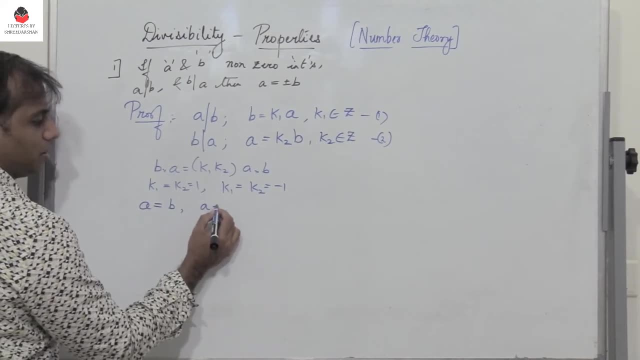 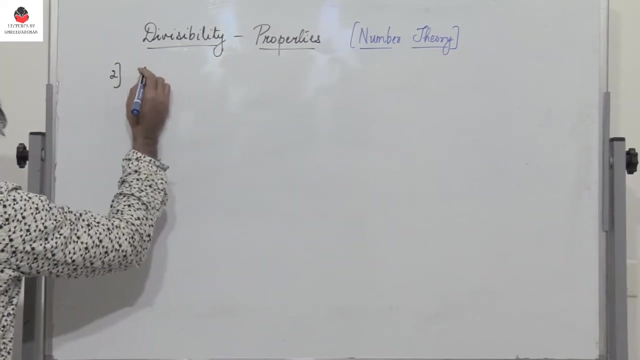 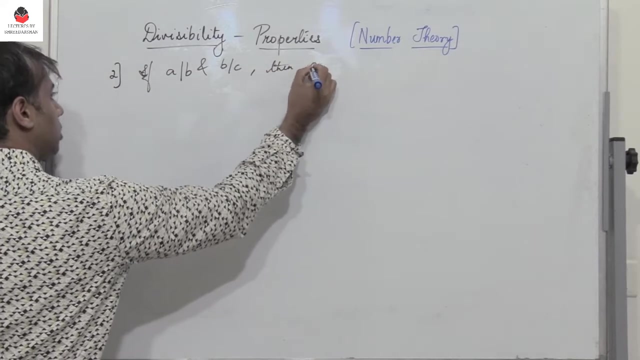 or K1 is equal to K2 is equal to minus 1.. Or we can say that A is equal to B or A can be equal to minus B. So therefore we say that A is equal to plus or minus B, The second property. if A divides B and B divides C, then we conclude that A divides C. 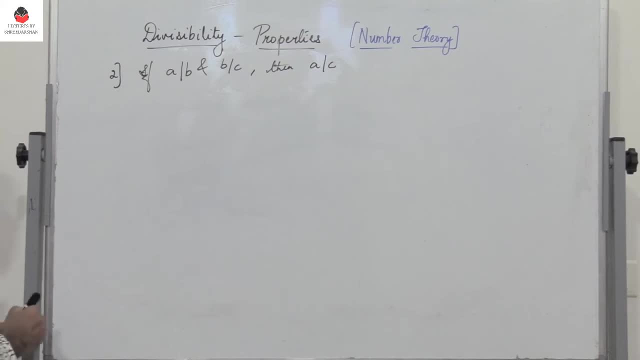 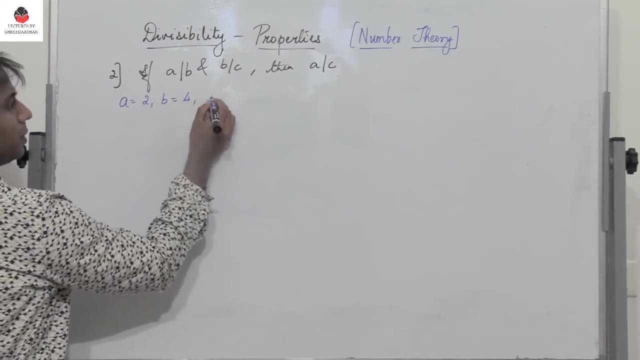 Now, how do we prove this? So let us first take an example. Now, if A is equal to 2 and B is equal to 4. And then if I have C, then I have A is equal to 2.. So let us first take an example. 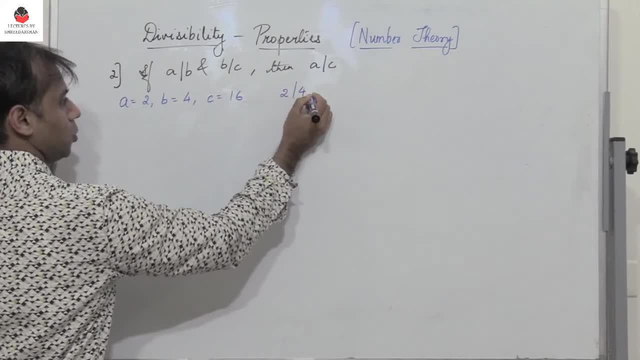 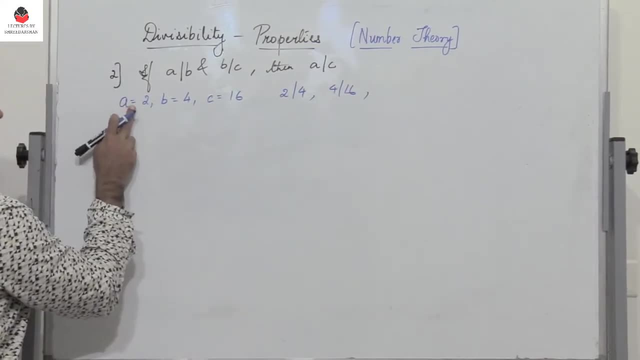 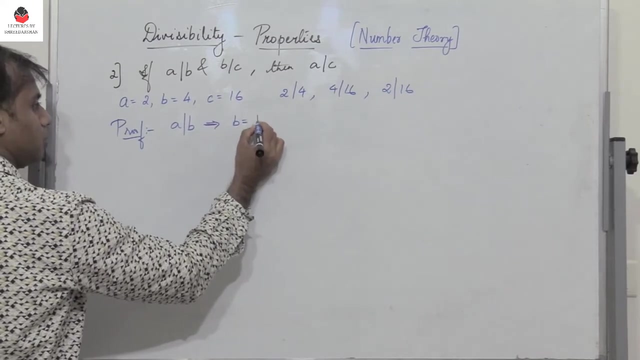 B is equal to 16.. We know that 2 divides 4.. And here we have 4 divides 16, which is B divides 16.. And also A divides 16.. So 2 divides 16.. A divides B, which implies that B is equal to K1 into A. 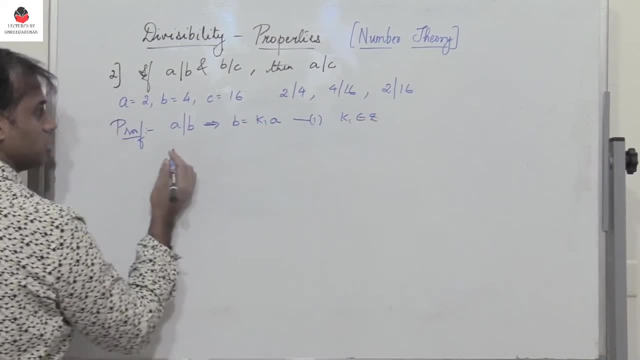 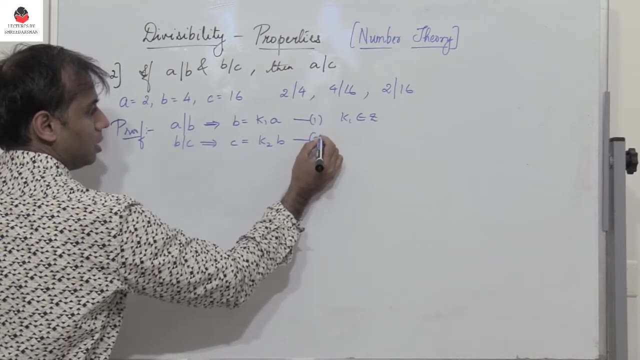 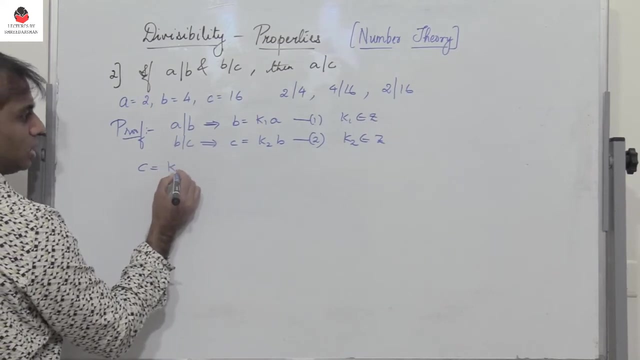 Call this as: 1, where K1 belongs to the set of integers. So similarly, B divides C, which implies E equation 2, where K2 belongs to Z Right. So C equals K2 into B. But what is B? B is nothing but. 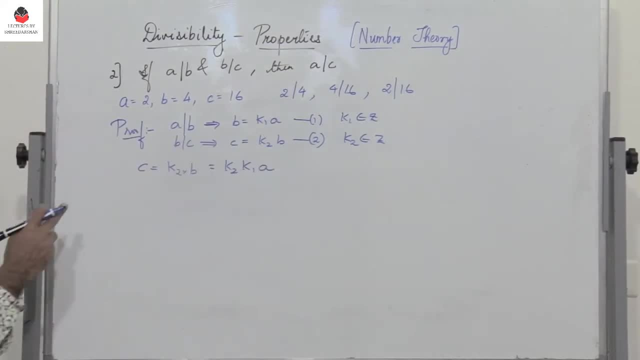 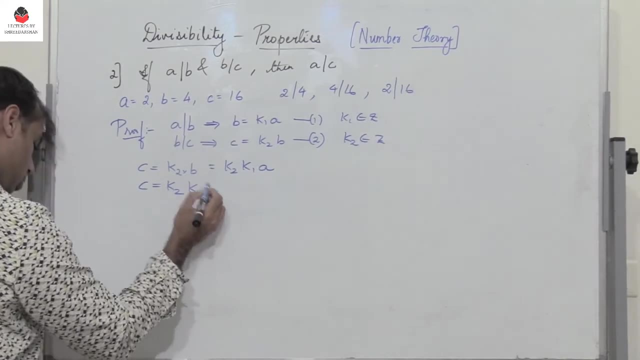 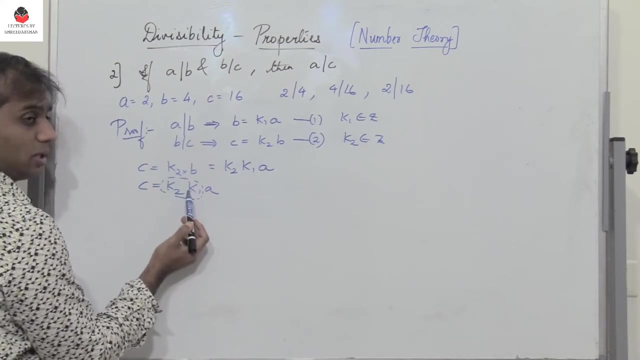 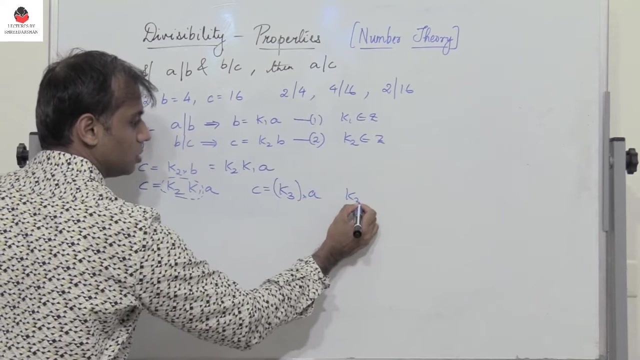 K1 into A Right. So therefore here I have C equals K2 into K1, K2 into K1 into A. Now can I call this as another value K3, because K1 is an integer is an integer. You multiply two integers, you get another integer, k3.. So k3 into a, where k3 also. 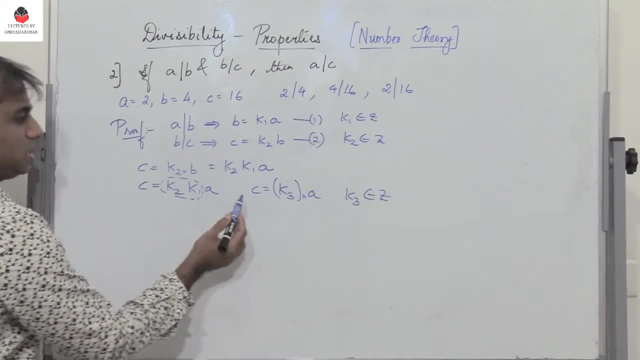 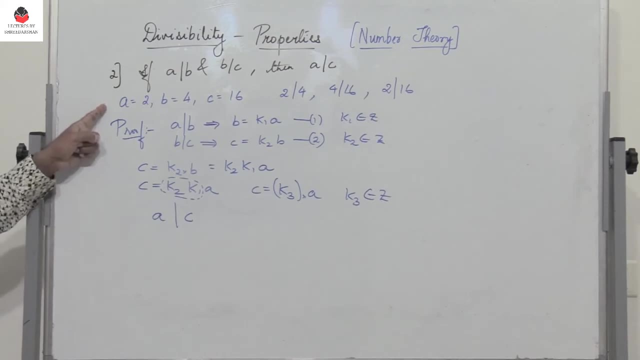 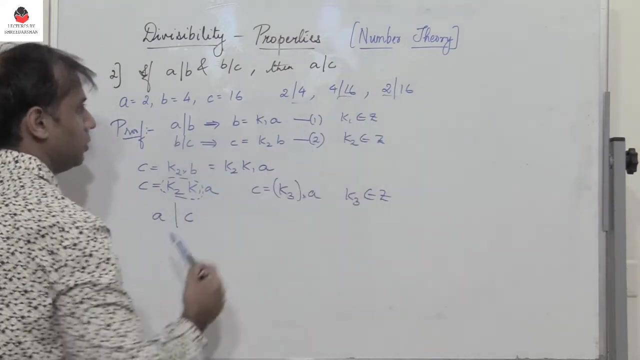 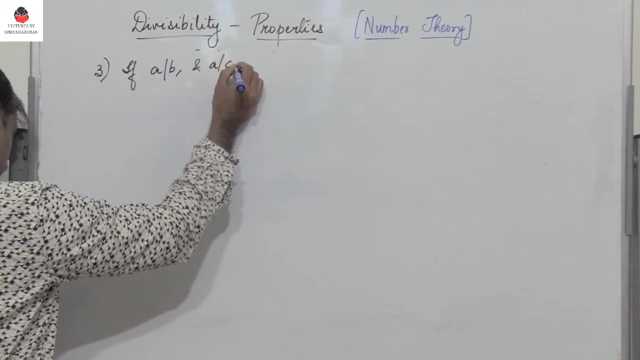 belongs to the set of integers. So if c equals k3 into a, then definitely a divides c. So we have already taken an example and we have shown that if a divides b and if b divides c, therefore a will definitely divide c. 3, if a divides b and if a divides c, then we have three relations: a divides- 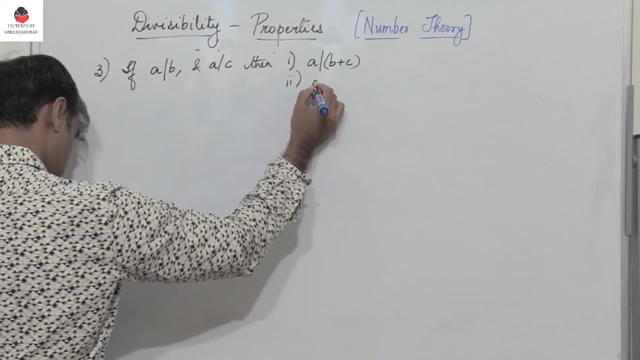 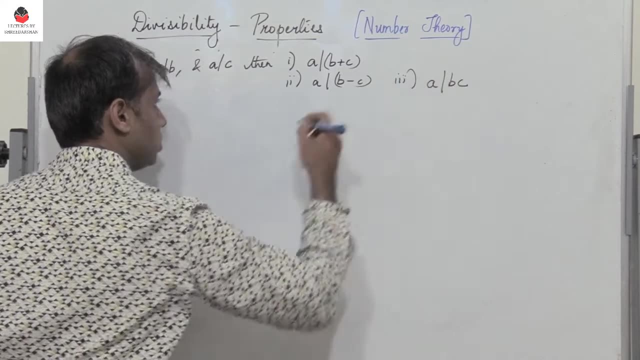 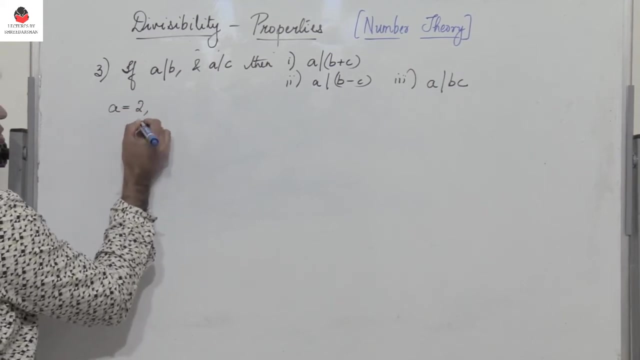 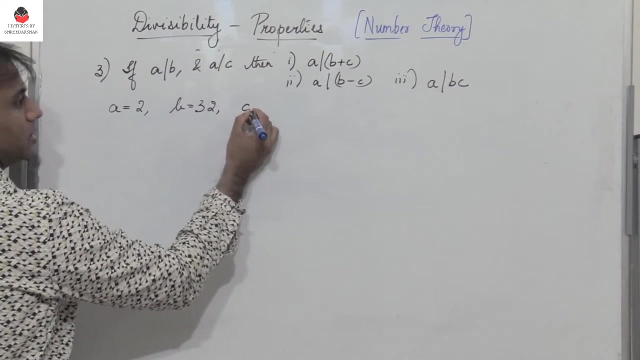 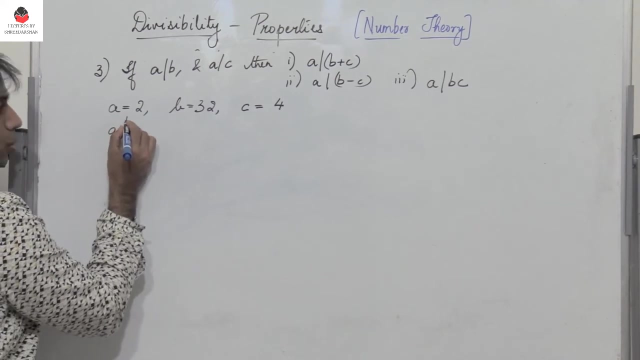 b plus c, 2, a divides b minus c and 3, a divides b into c, right? So let's take a few examples. So let a be equal to 2.. Let b be equal to 32 and let c be equal to 4.. Now here we observe that a divides. 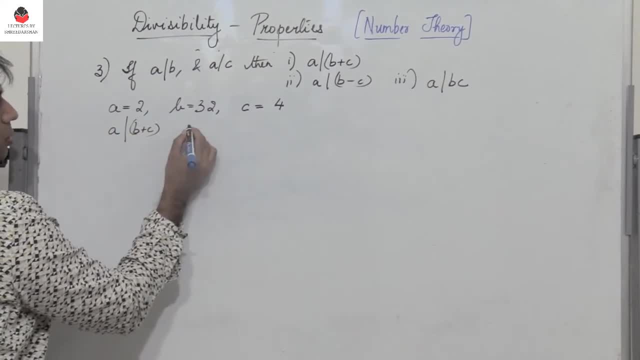 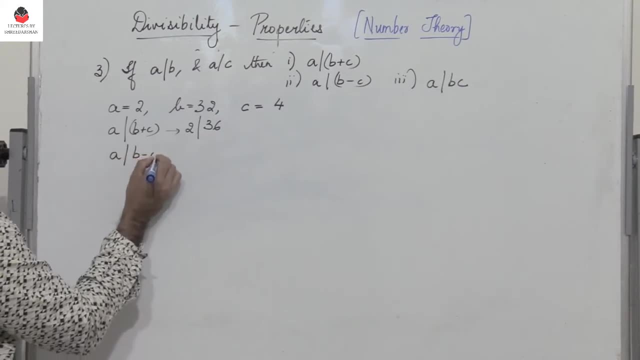 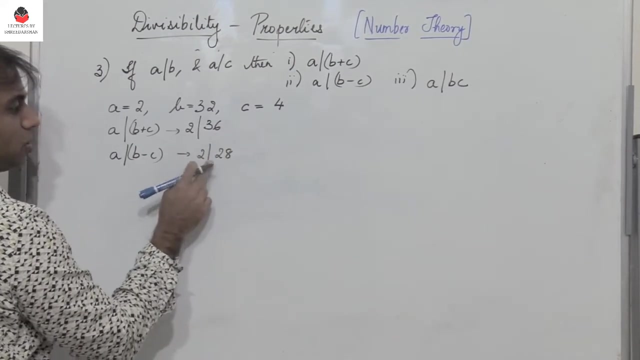 b plus c. So let me write the value Now: 2 definitely divides 32 plus 4, which is 36.. Next, a divides b minus c, which implies 2 divides 32 minus 4, which is 28.. So definitely 2 divides. 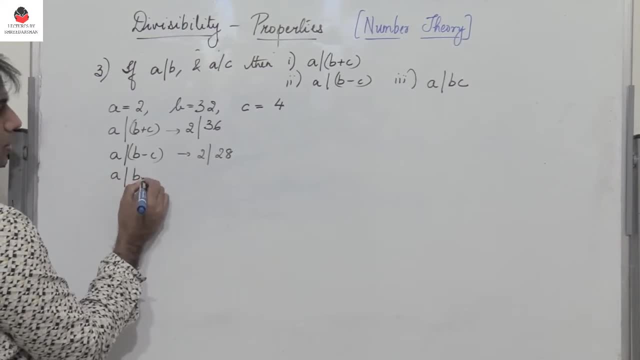 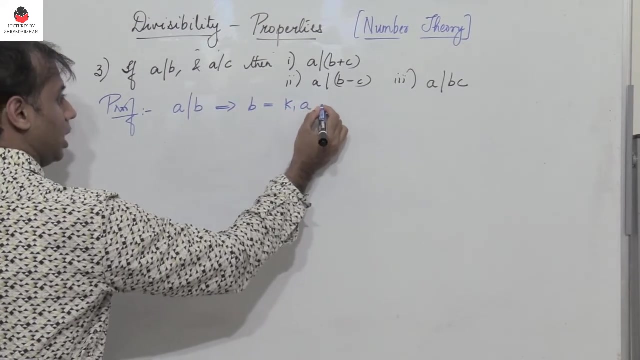 28.. Now a definitely will divide b into c. So 2 divides 32 into 4 definitely. So we have taken an example. So let us prove this. a divides b implies b is equal to k1 into a. So call this: 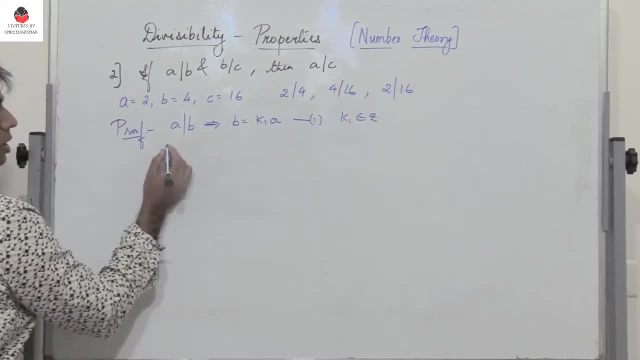 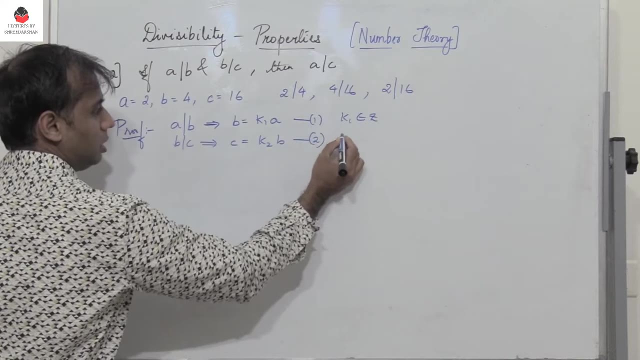 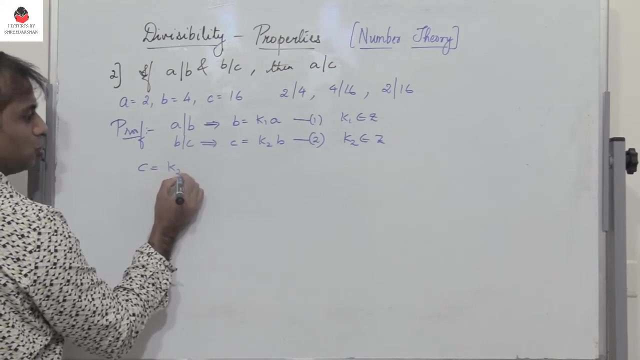 as 1, where K1 belongs to the set of integers. So similarly, B divides C, which implies that C is equal to K2 into B. Equation 2, where K2 belongs to Z, So C equals K2 into B. But what is B? B is nothing but K1. 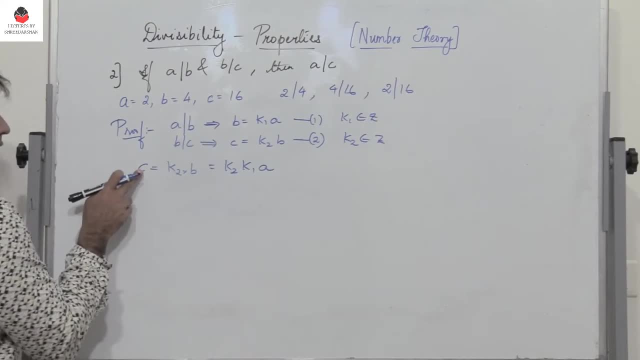 into A. So therefore, here I have C equals K2 into K1, K2 into K1 into A. Now can I call this as another value, K3, because K1 is an integer, K2 is an integer. So here I have C equals K2 into K1, into. 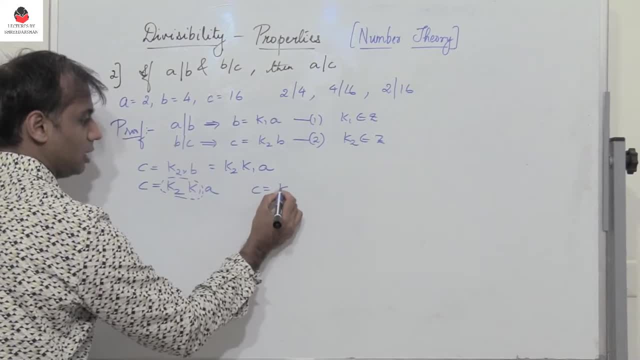 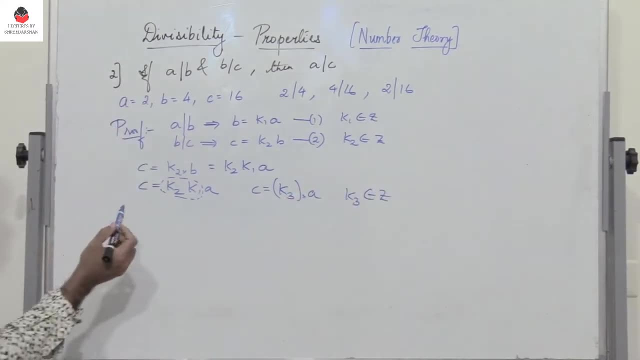 K2 is an integer. You multiply two integers, you get another integer, K3.. So K3 into A, where K3 also belongs to the set of integers. So if C equals K3 into A, then definitely A divides C. So we have. 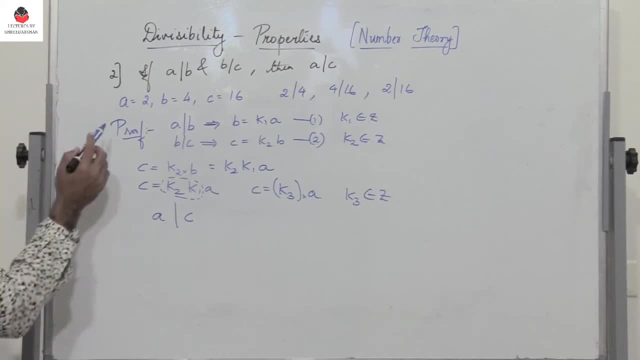 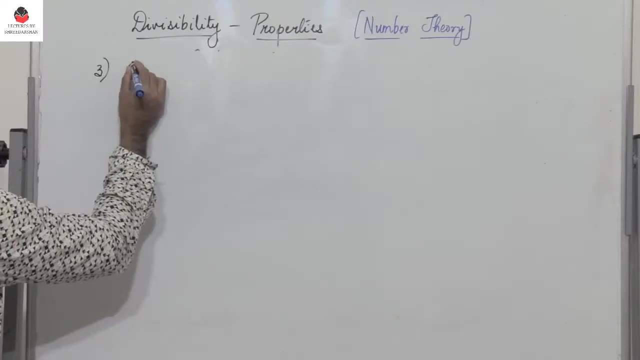 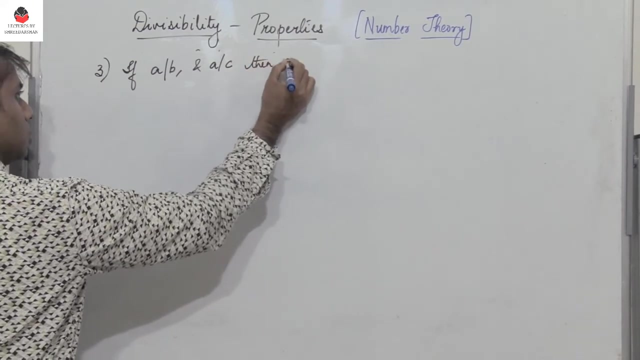 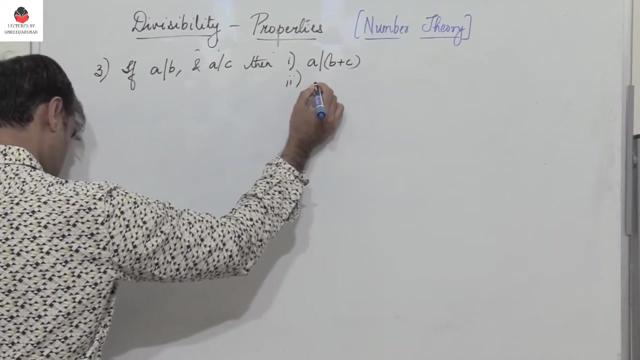 already taken an example and we have shown that if A divides B and if B divides C, therefore A will definitely divide C. 3. If A divides B and if A divides C, then we have three relations: A divides B plus C, 2. A divides B minus C And 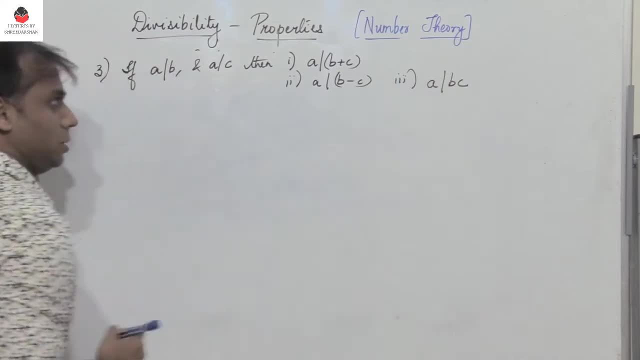 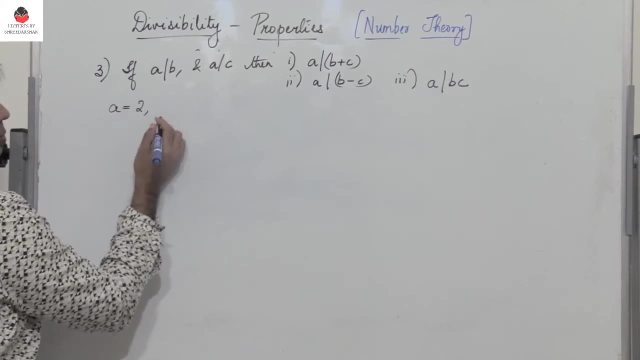 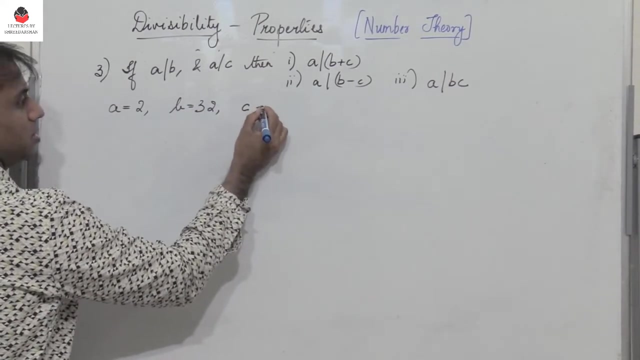 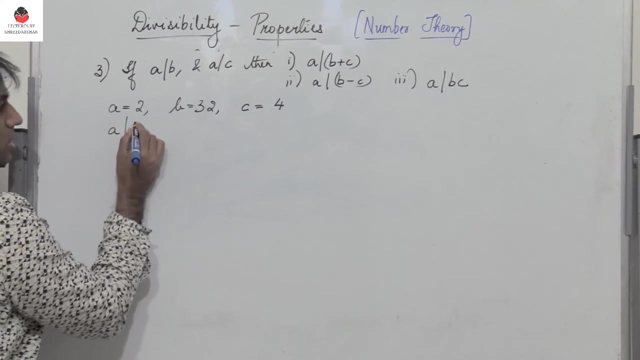 3. A divides B into C. So let us take a few examples. So let A be equal to 2. Let B be equal to 32. And let C be equal to 4.. Now here we observe that A divides B plus C. So let me write the value Now. 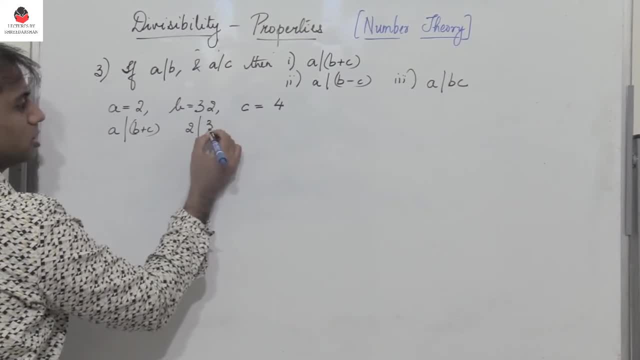 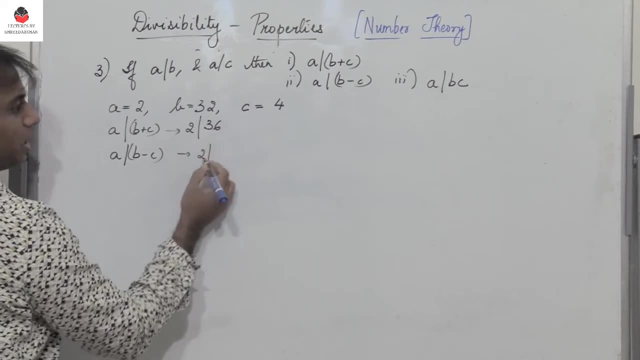 2 definitely divides 32 plus 4,, which is 36.. Next, A divides B minus C, which implies 2 divides 32 minus 4, which is 28.. So definitely 2 divides 28.. Now A definitely divides 32 plus 4,, which is 28.. 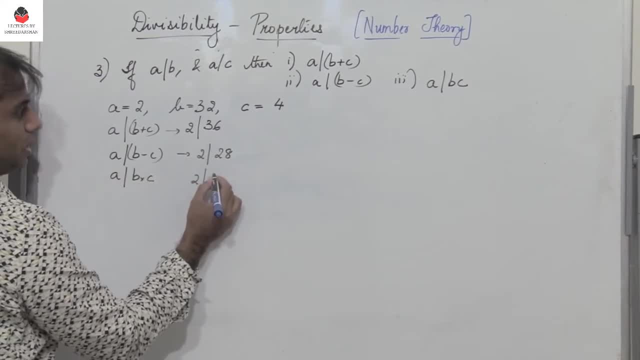 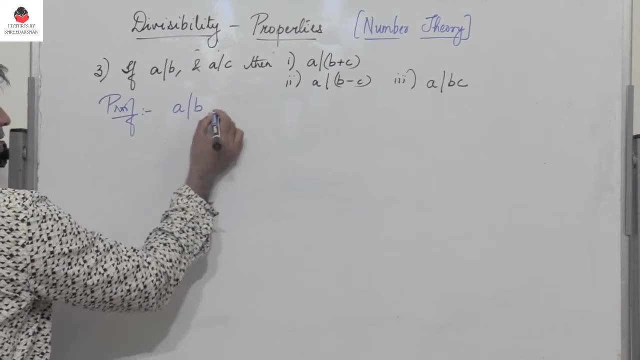 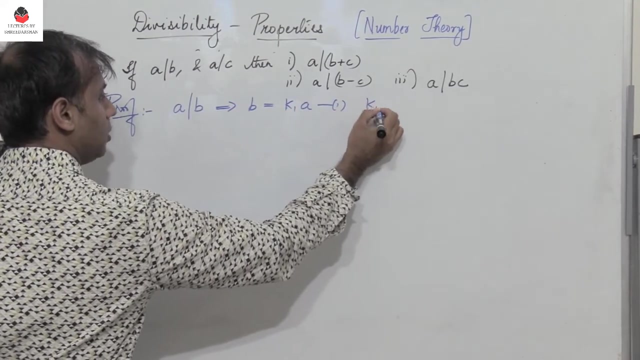 So 2 definitely will divide B into C. So 2 divides 32 into 4, definitely. So we have taken an example. So let us prove this. A divides B implies B is equal to K1 into A. So call this as 1, where K1. 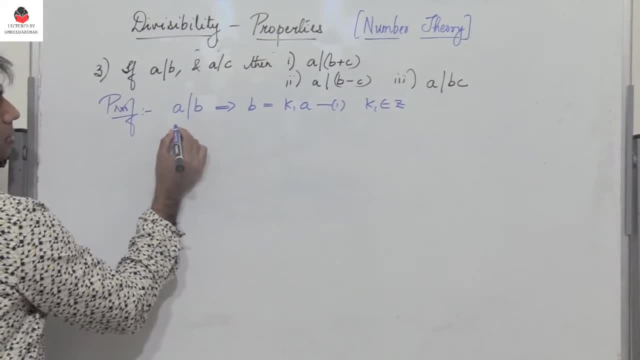 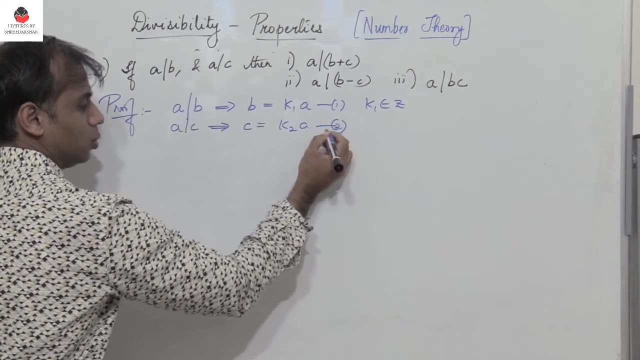 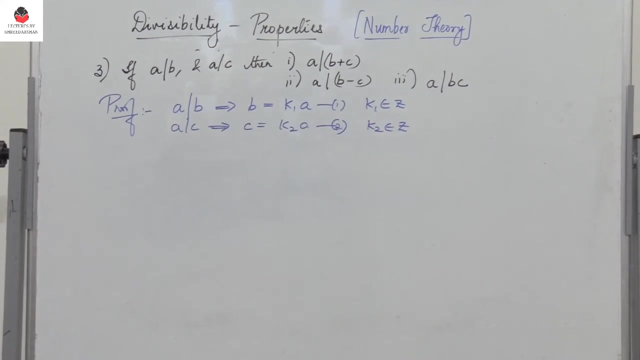 belongs to the set of integers Z. Similarly, A divides C, which implies that C equals K2 into A, which is equation 2, where K2 belongs to the set of integers Z. Now let me add 1 and 2.. When you add 1 and 2,, 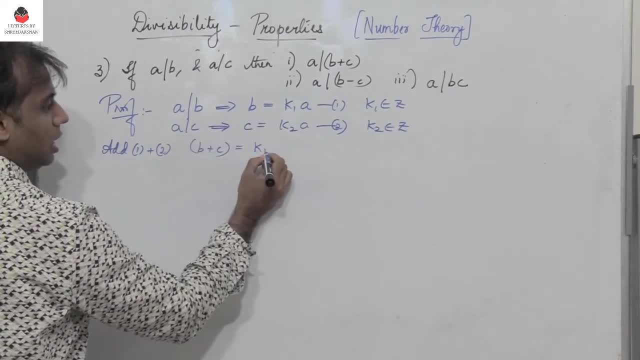 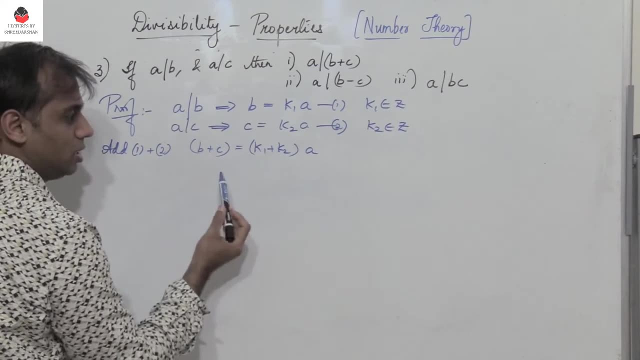 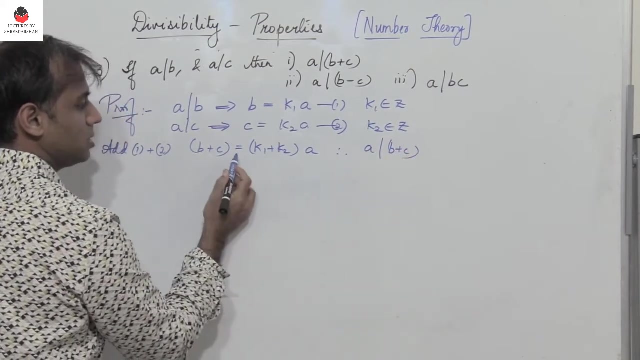 you get B plus C- equals K1 plus K2- into A. Now, since K1 and K2 are integers, K1 plus K2 is also an integer, And therefore here we have A divides B plus C, because B plus C 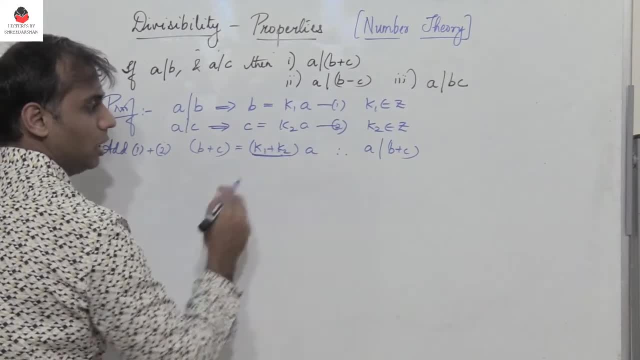 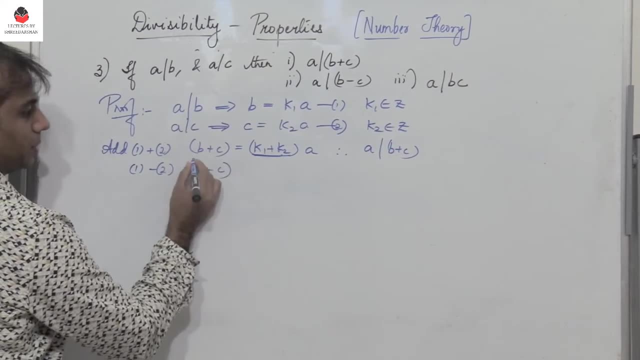 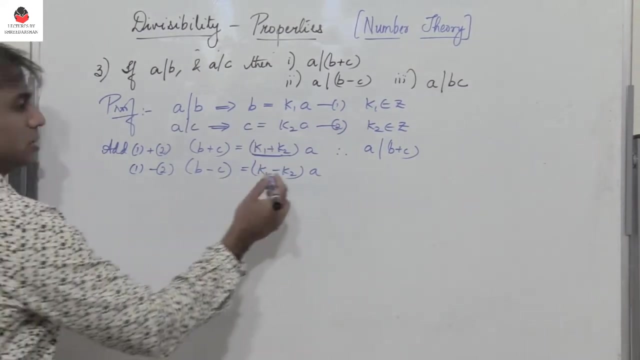 equals K1 plus K2 into A. So therefore A divides B plus C. Next perform subtraction 1 minus 2. So you get B minus C equals K1 minus K2 into A. So again, K1 minus K2 is an integer. So therefore: 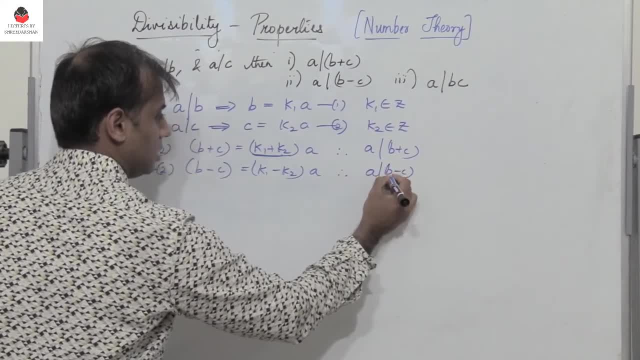 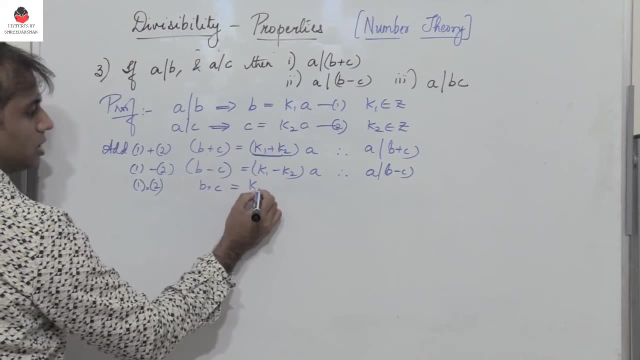 we can conclude that A divides B minus C, And then the next one multiply 1 and 2.. So we get B into C equals K1 into K2.. So we get B minus C equals K1 minus K2 into A. So again, K1 minus K2 is an integer. So 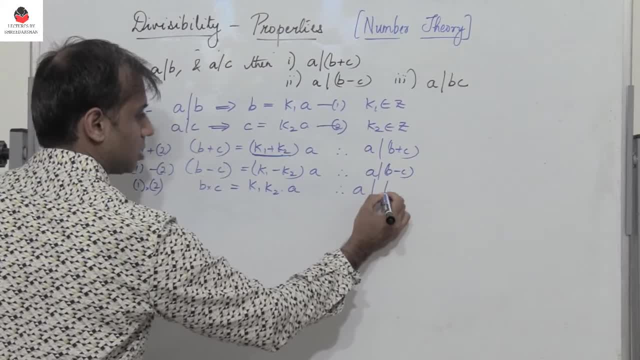 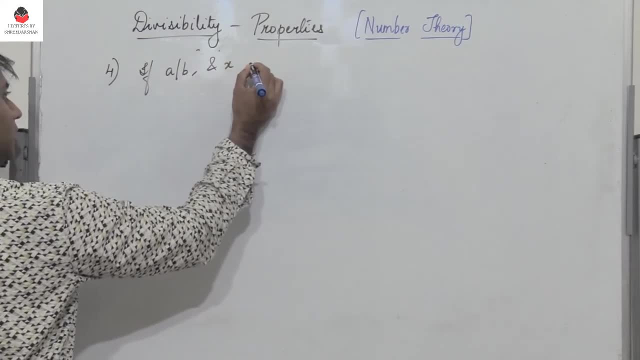 we get B minus C equals K2 into A. So again, K1 minus K2 is an integer. So we get B minus C equals K2 into A, And therefore A divides B into C. Very simple proof: If A divides B and X is any integer, then A divides. 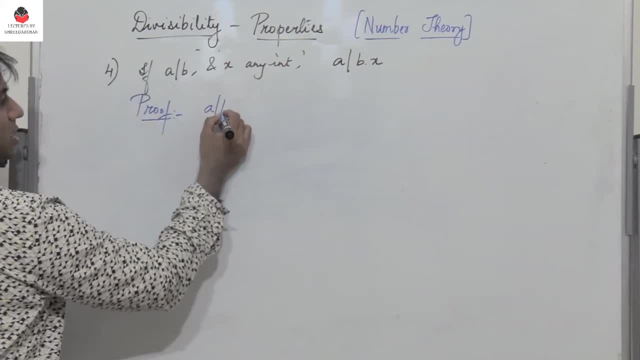 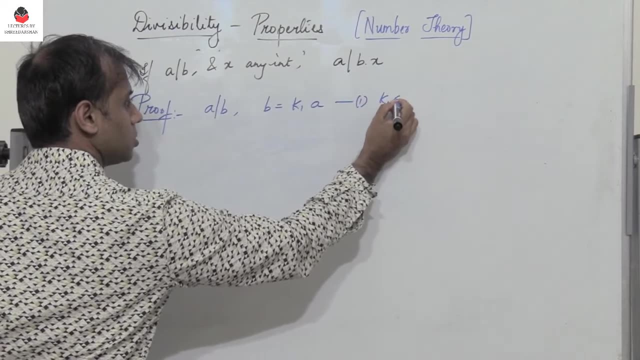 B into X. So proof A divides B, which means B is equal to K1 into A. So let me call this as 1, where K1 belongs to a set of integers. Now multiply equation 1 on both the sides with X. So 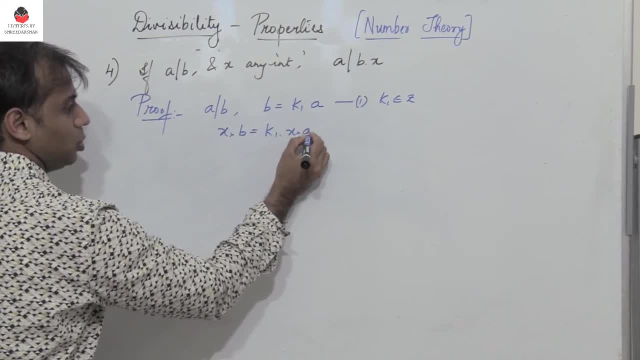 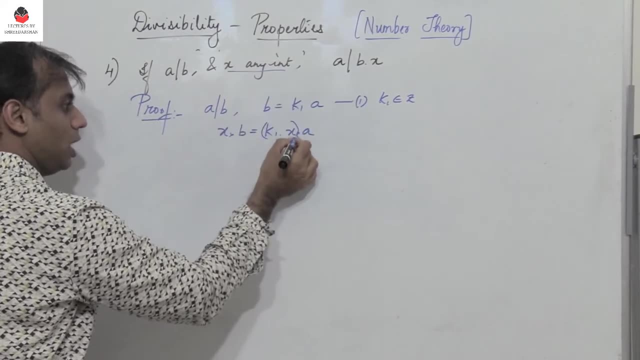 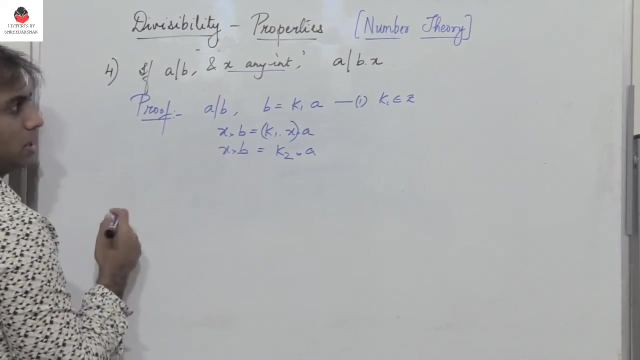 we get A into B equals K1 into X into A. Now K1 is an integer, X also is an integer which has been given. So K1 into X can be written as K2 into A. So you have X into B. So X into B is equal to K1. 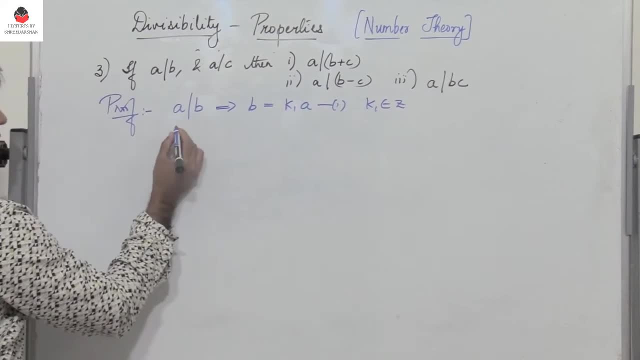 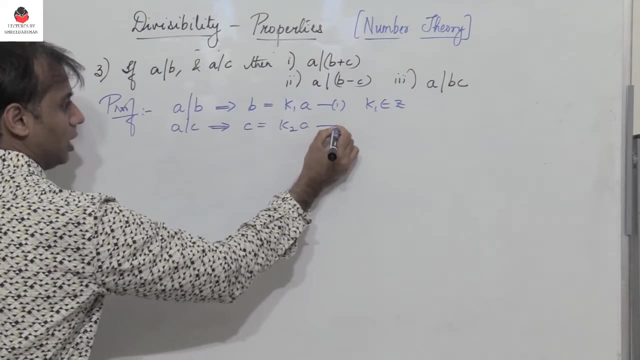 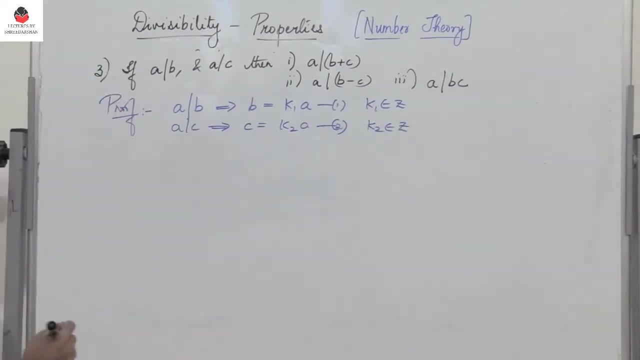 1, where k1 belongs to a. So let us prove this. So let us prove this. So let us prove this: k1 belongs to the set of integers z. Similarly, a divides c, which implies that c equals k2 into a, which is equation 2, where k2 belongs to the set of integers z. Now let me add 1 and 2.. When you 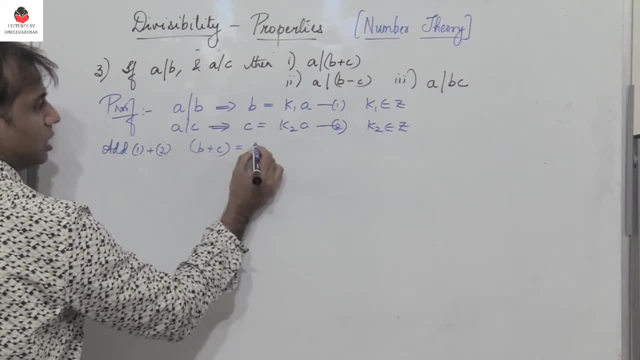 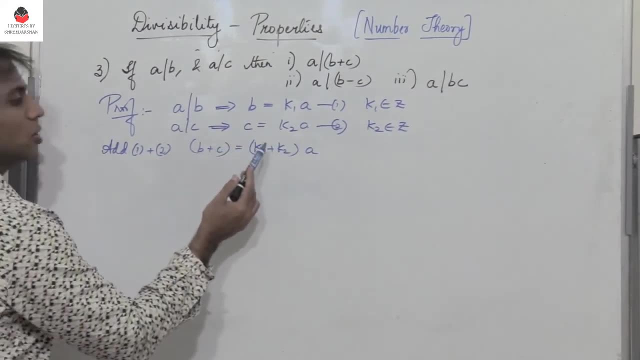 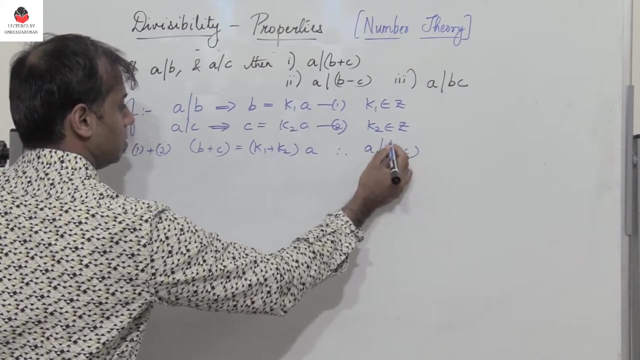 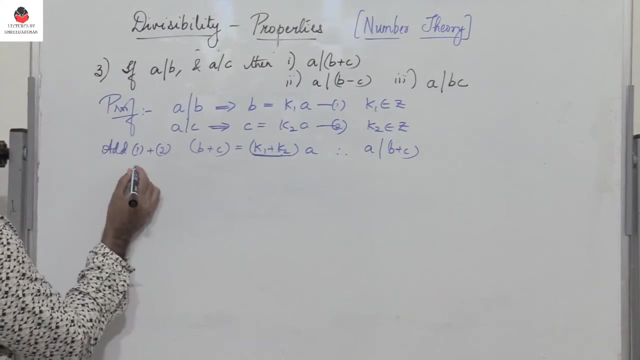 add 1 and 2, you get b plus c- equals k1 plus k2- into a. Now, since k1 and k2 are integers, k1 plus k2 is also an integer and therefore here we have a divides b plus c, because b plus c equals k1 plus k2 into a. So therefore a divides b plus c. Next perform: 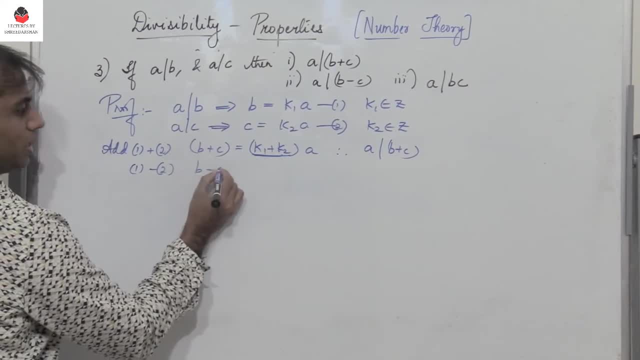 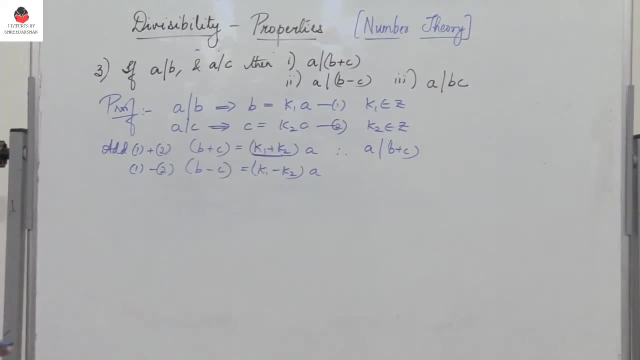 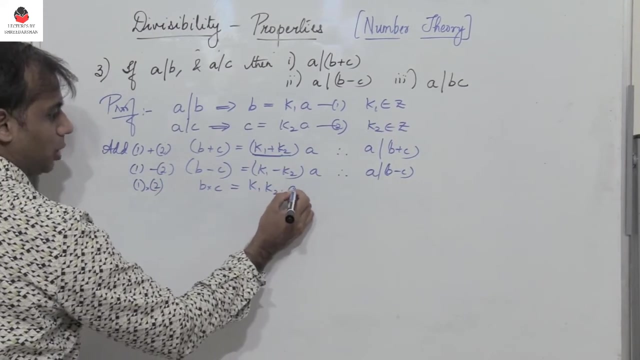 subtraction 1 minus 2. So you get b minus c equals k1 minus k2 into a. So again, k1 minus k2 is an integer. So therefore we can conclude that a divides b minus c, And then the next one multiply 1 and 2.. So we get b into c, equals k1 into k2 into a. 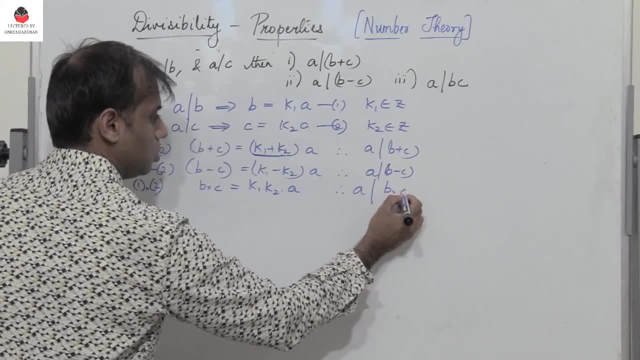 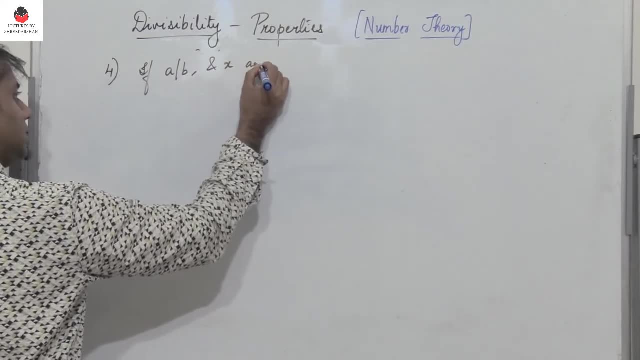 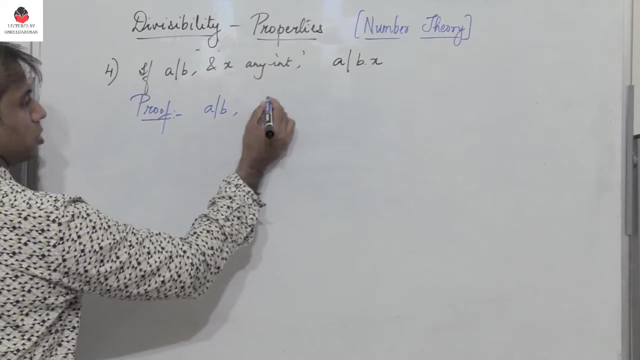 and therefore a divides b into c. Very simple proof. If a divides b and x is any integer, then a divides b into x. So proof: a divides b, which means b is equal to b. So if you think the same thing is true, then the same thing is true and gradually it. Pi should be. 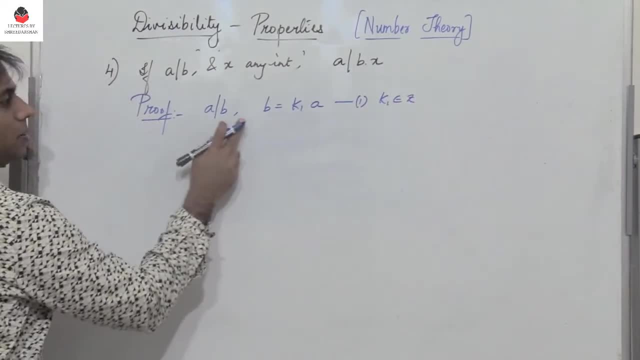 naughty. Now imagine that we draw a b into it. So it writes b as a integer. but here we run to our data that b is equal to c, which is a set of integers- JSON time, And this would be b over integral 0.. Now we will spend a little more time on the same thing. We will punch this. 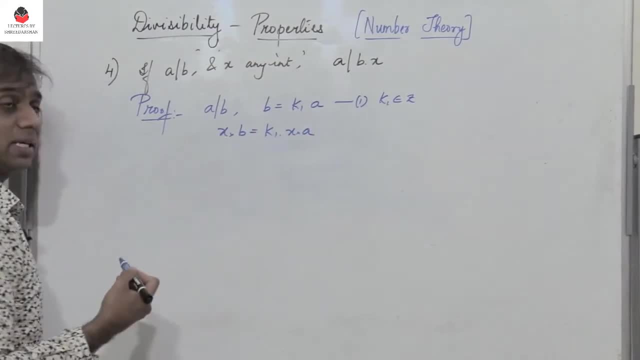 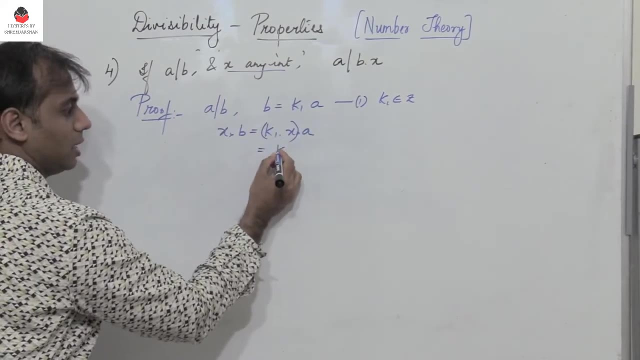 uria filter in a way. So actually there are some possible places to add the sign Lincoln. So these are all the states. So again, we're going to write k into a as C equal to 1.. Let's play that for everyone. watch carefully, then we can do this work. I'm going to calculate the. 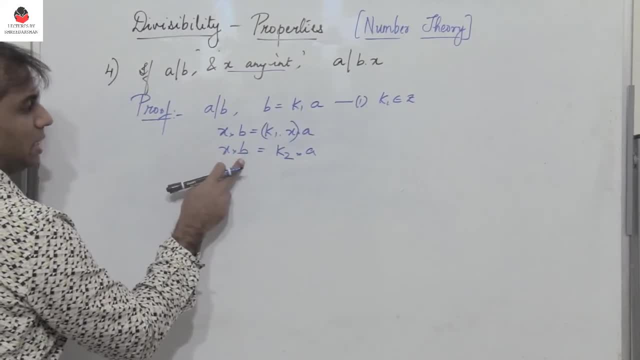 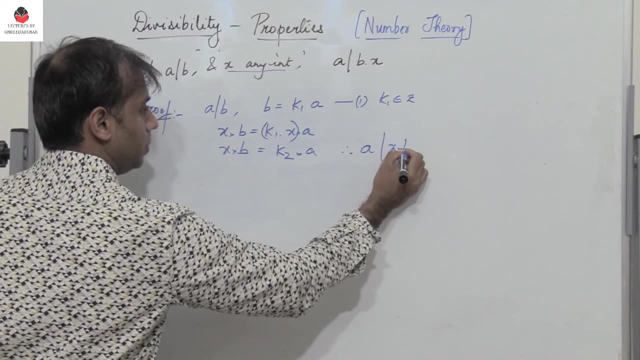 Sanskrit notation for the mange, and this is the same as the Sin Network. so sine k1 sus with the average kesares, that is minus a into A. So let me call this as 1, where So x into b is equal to k1 into a. So therefore we can conclude that a divides x into b or a. 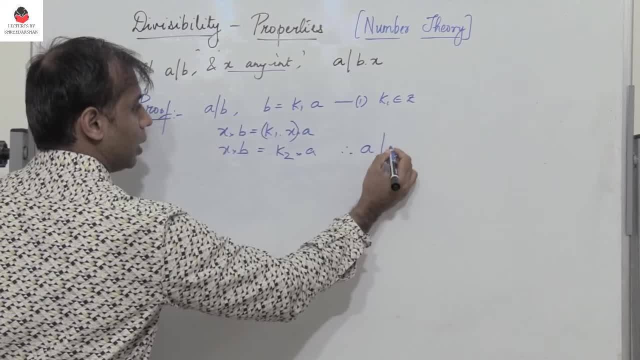 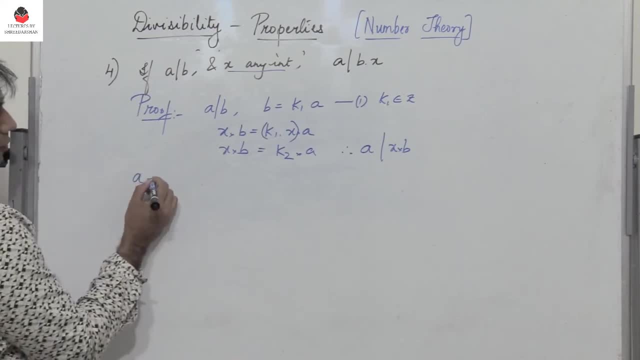 into A. So therefore, we can conclude that A divides X into B or A divides B into X. So let's take an example: If A is equal to 2, and if B is equal to 8,, we know that A divides B, 2 divides 8.. Now here: 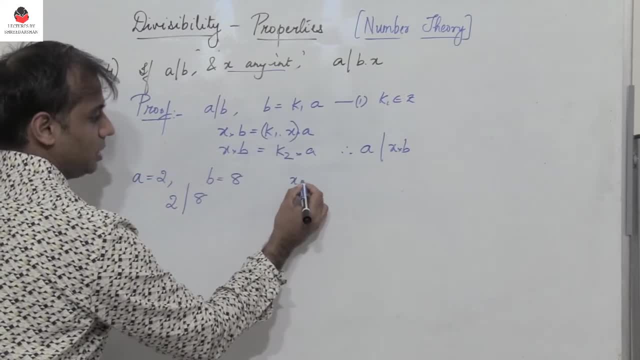 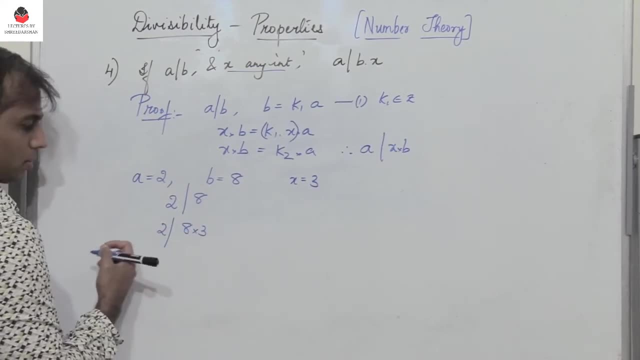 multiply both B and A with a value X, So let X be 3.. So therefore A, 2, will definitely divide 8 into 3, which is 24.. So here we realize that if I multiply B with any integer X, A will definitely. 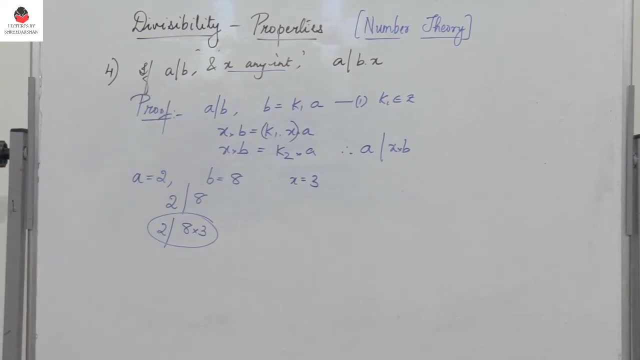 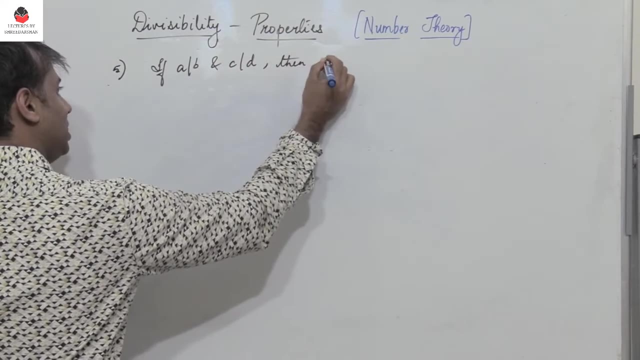 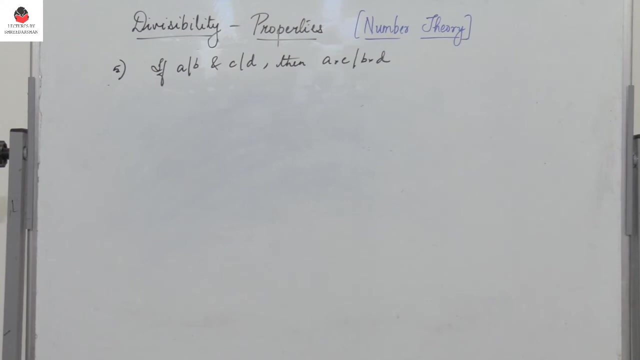 divide B into X, If A divides B and if C divides D, then A into C will definitely divide B into D. So again, this is a very simple proof. So before we see the proof, let's take a few examples. Now, here I have 2. 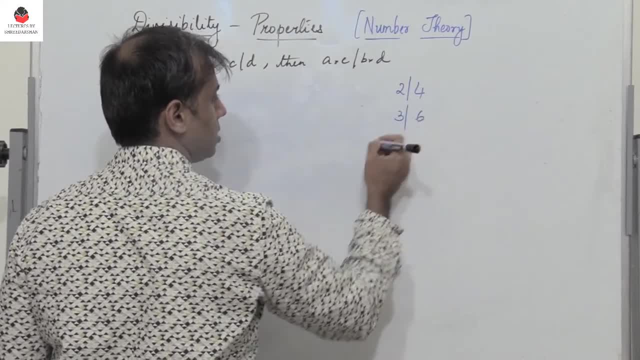 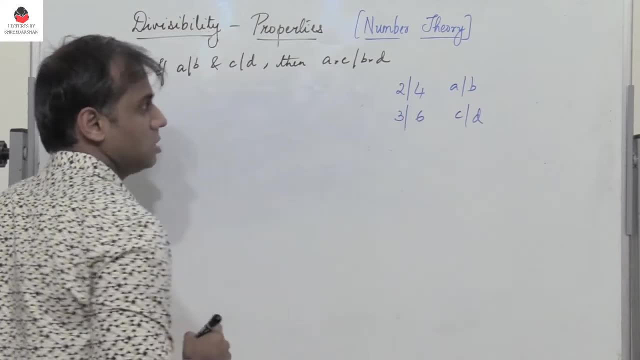 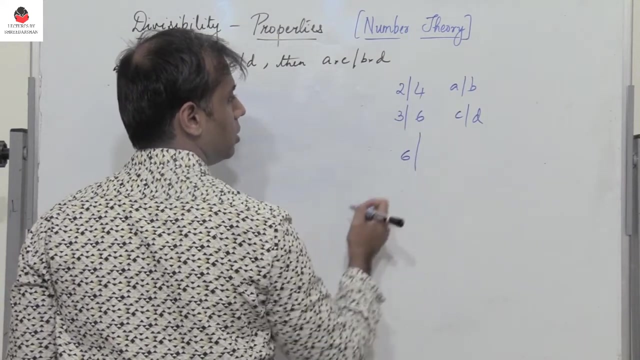 divides 4, and 3 divides 6.. So this is A divides B, and so this is C divides B. So here I have 2 divides D. So let me multiply A into C. What is A into C? 2 into 3,, which is 6.. Will it divide 6 into? 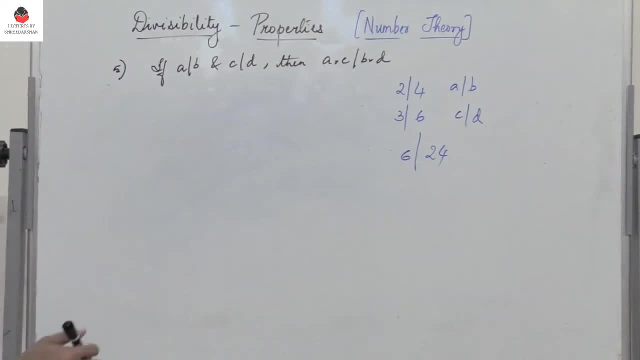 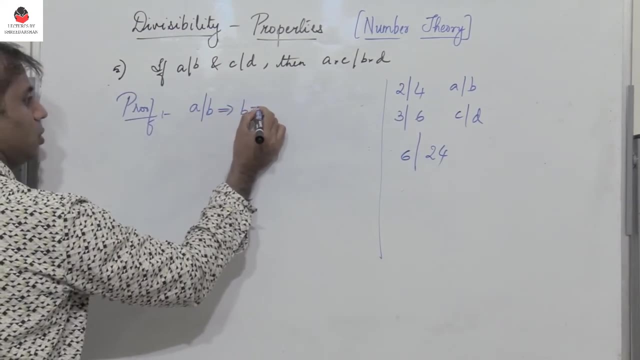 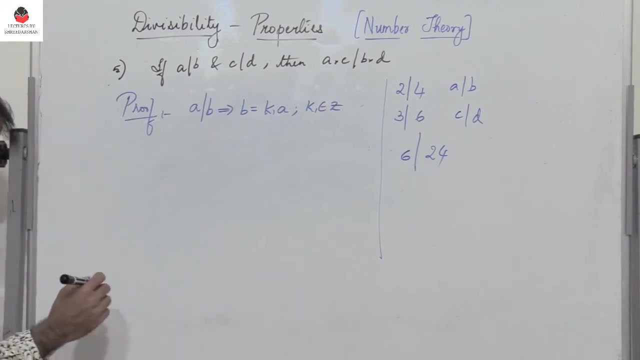 4? 24, yes, So 6 divides 24.. So you can take a number of examples. So let's see the proof Now. here: A divides B, which implies B equals K1 into A, where K1 is an integer, belongs to a set of. 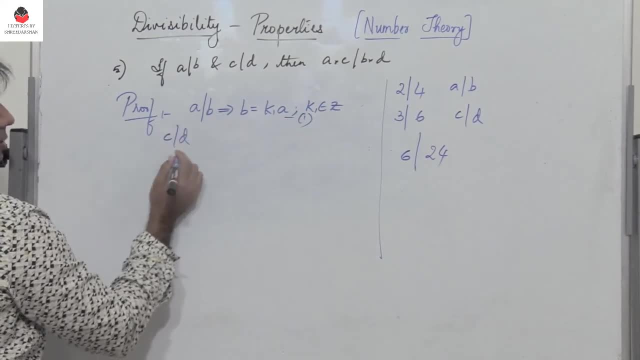 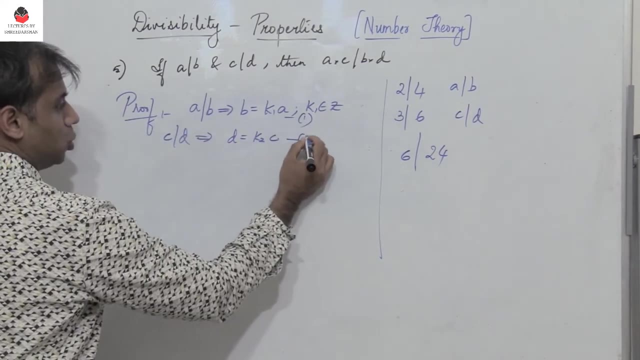 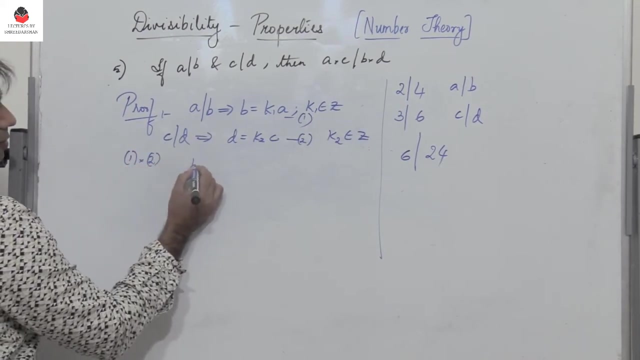 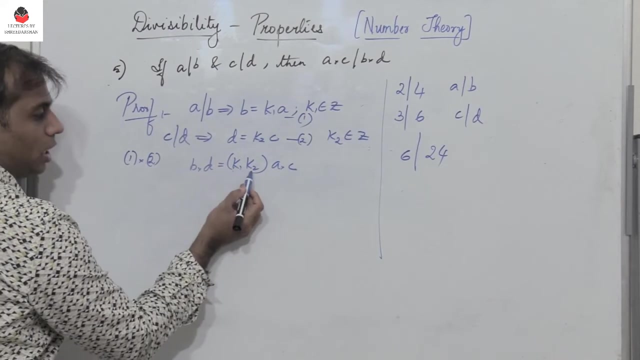 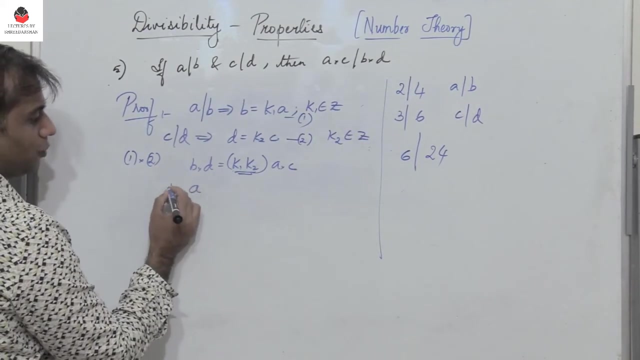 integers. Call this as 1. Now multiply 1 and 2. So you have B into D, equals K1 into K2 into A into C. So K1 into K2 is again an integer. because K1 is an integer, K2 also is an integer. So therefore we conclude that: 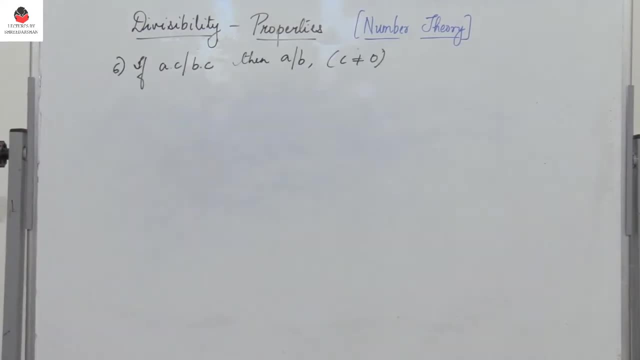 A into C divides B into D. So 6th one: if A into C divides B into C, then A divides B if C is not equal to 0. Again, it's a very easy proof here. So before we see the proof, let us take a few. 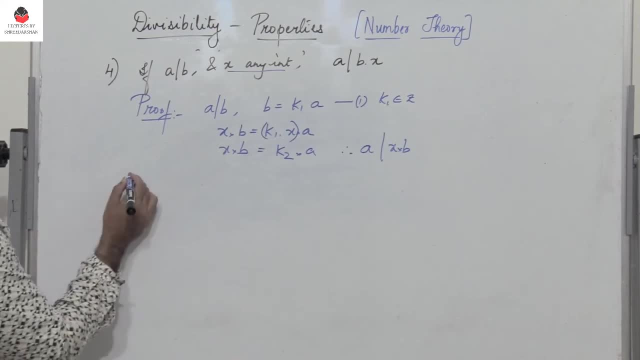 divides b into x. So let's take an example: If a is equal to 2 and if b is equal to 8, we know that a divides b, 2 divides 8.. Now here, multiply both b and a with a value x. So let x be 3.. 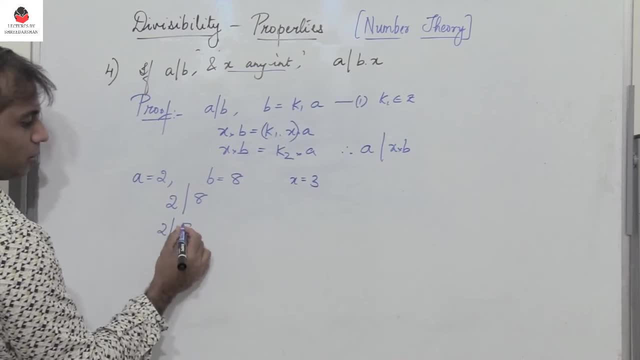 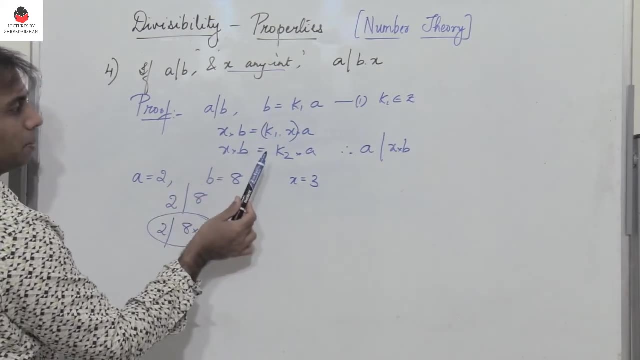 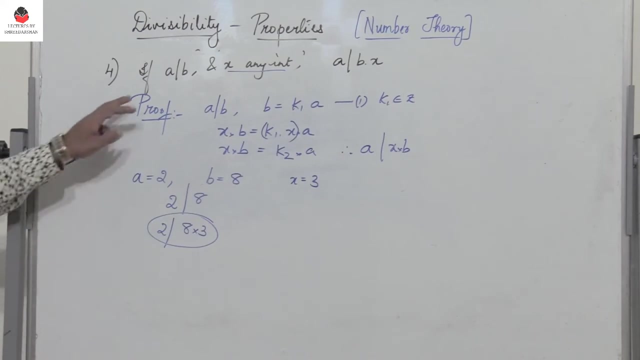 So therefore, a, 2 will definitely divide 8 into 3, which is 24.. So here we realize that if I multiply b with any integer, x, a will definitely divide b into x. if a divides b. If a divides b. 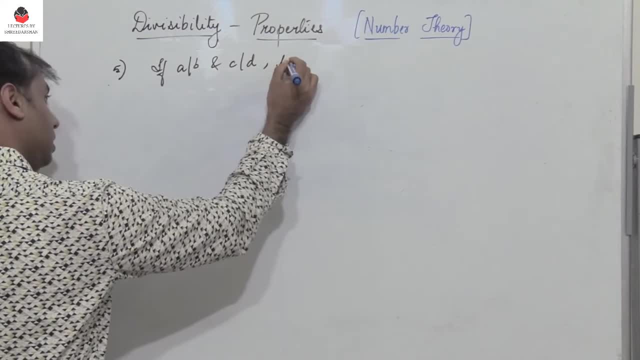 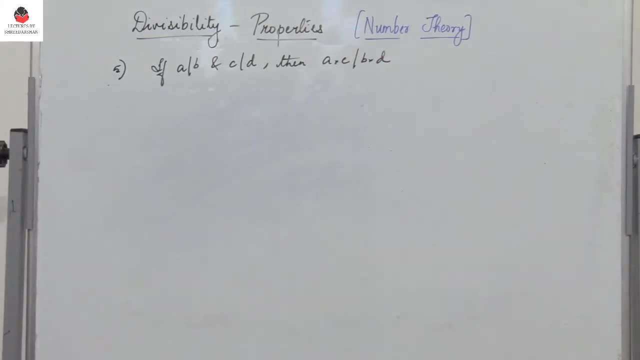 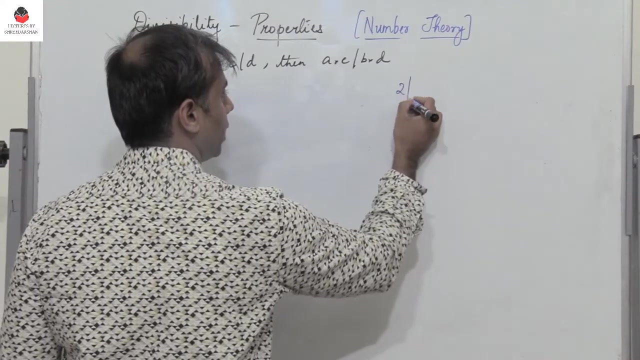 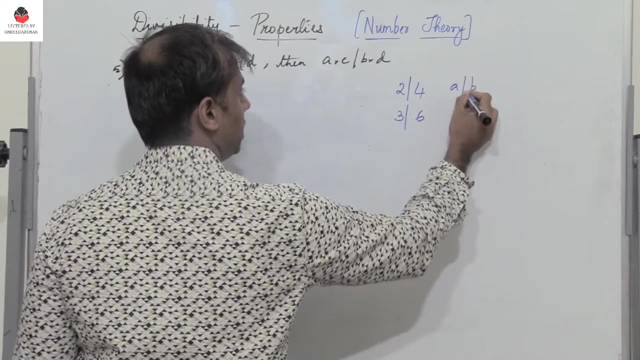 and if c divides d, then a into c will definitely divide b into d. So again, this is a very simple proof. So before we see the proof, let's take a few examples Now. here I have 2 divides 4 and 3 divides 6. So this is a divides b, and so this is c divides d. 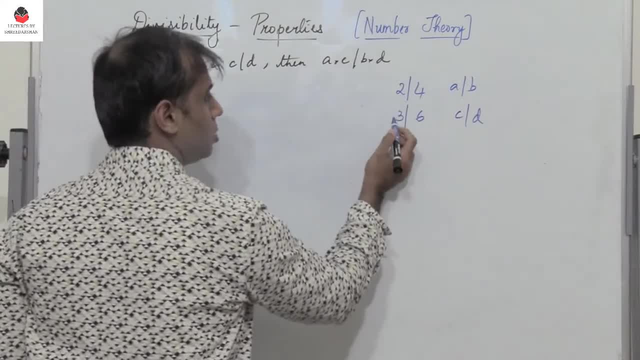 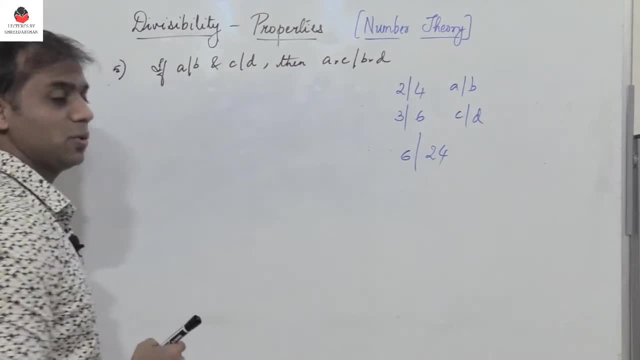 So let me multiply a into c, What is a into c, 2 into 3, which is 6.. Will it divide 6 into 4? 24, yes. So 6 divides 24.. So let's take a few examples. So let's take a few examples. So let's take a few examples. 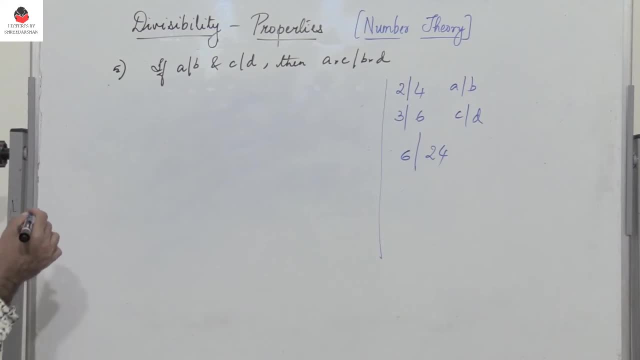 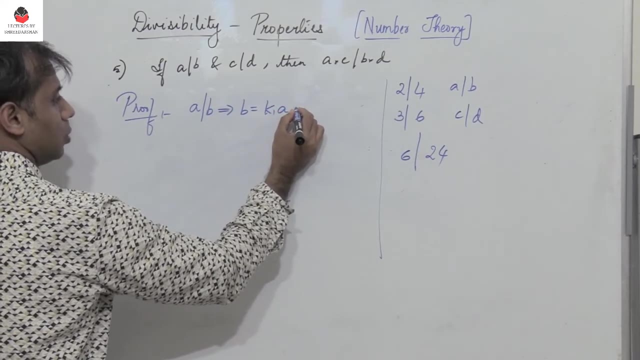 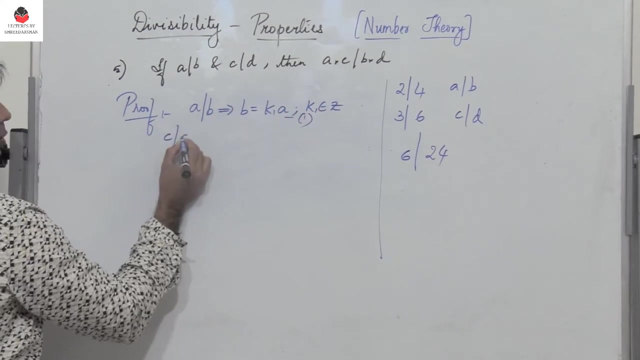 So you can take a number of examples. So let's see the proof Now here. a divides b, which implies b equals k1, into a, where k1 is an integer belongs to a set of integers. Call this as 1.. c divides d, which implies that d is equal to k2. 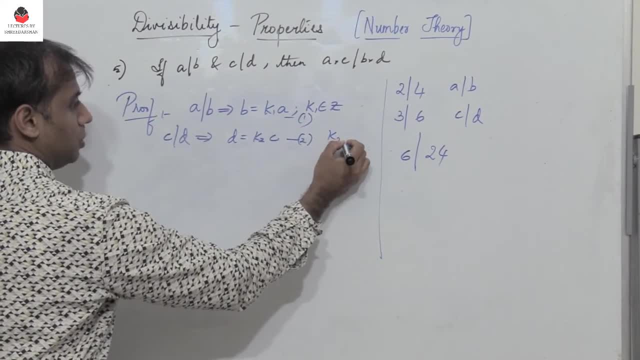 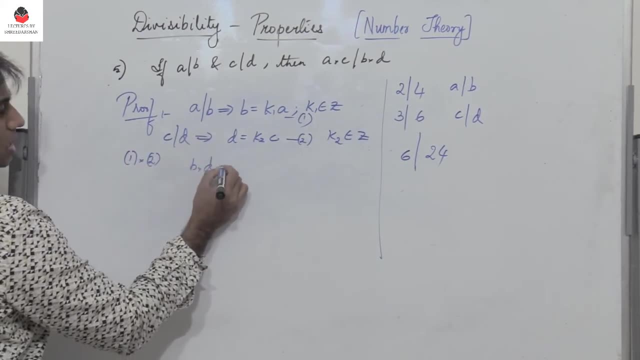 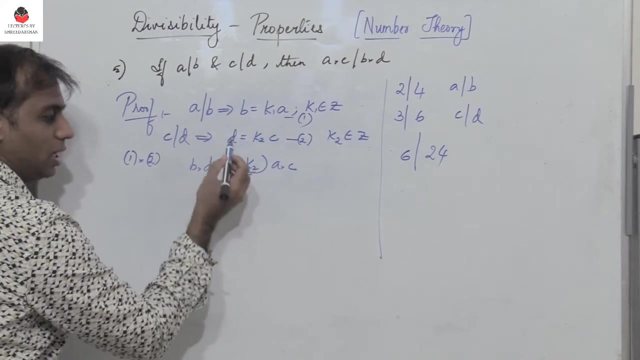 into c, So call this as 2, where k2 belongs to a set of integers. Now multiply 1 and 2. So you have b into d equals k1 into k2, into a into c. So k1 into k2 is again. 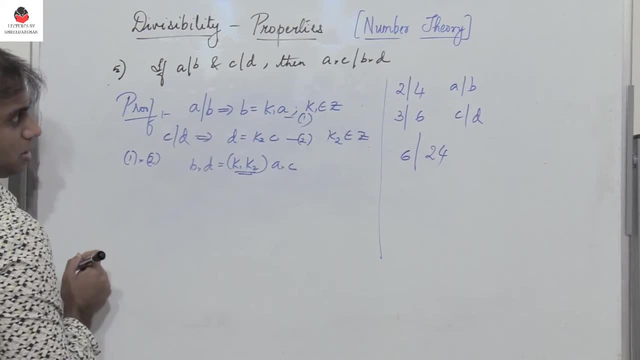 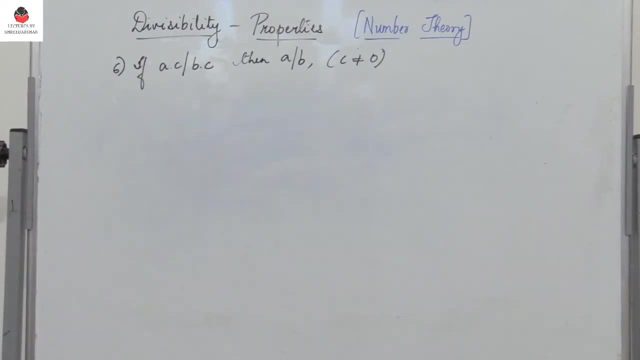 an integer, because k1 is an integer, k2 also is an integer. So therefore we conclude that a into c divides b into d. So sixth one: if a into c divides b into c, then a divides b. if c is not. 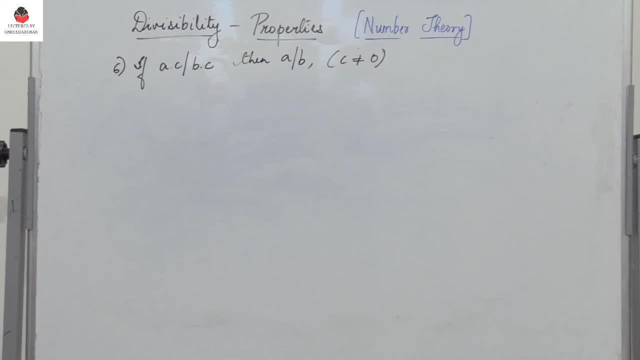 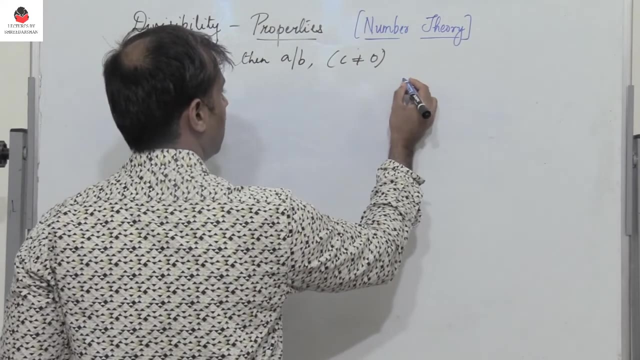 equal to 0.. Again, it's a very simple proof. So let's take a few examples. So let's take a few very easy proof here. So, before we see the proof, let us take a few examples. So I have 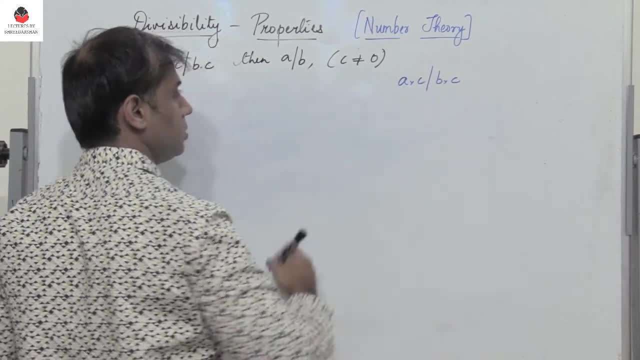 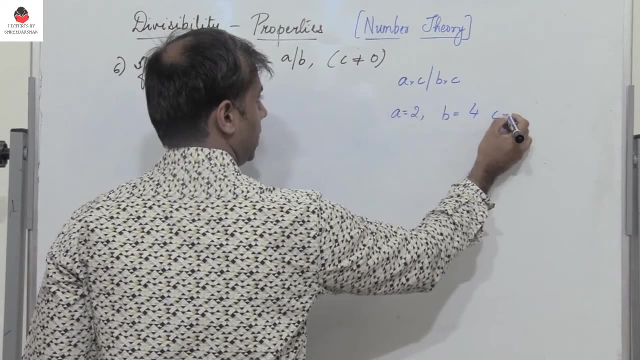 a into c should divide b into c. So let me take a to be equal to 2, b to be equal to 4, and let c be equal to 3.. So observe a into c, which is 6,, 2 into 3, is 6, divides b into c. 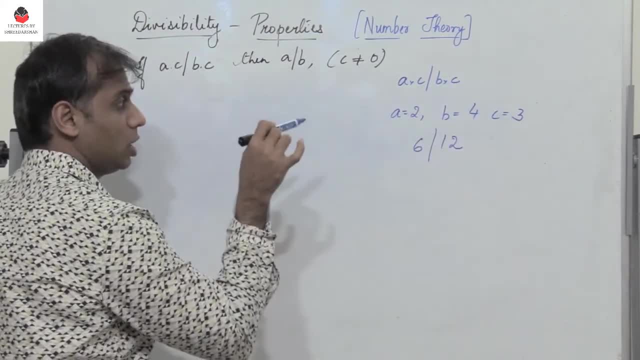 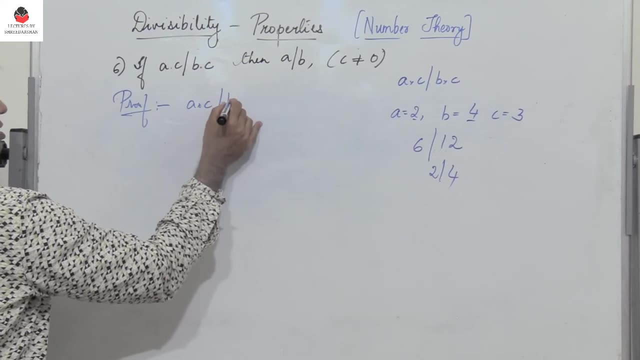 4 into 3, which is 12.. 4- 3s are 12.. Now, if that is the case, then definitely a divides b, 2 divides 4.. a into c divides b into c, which implies that b into c. 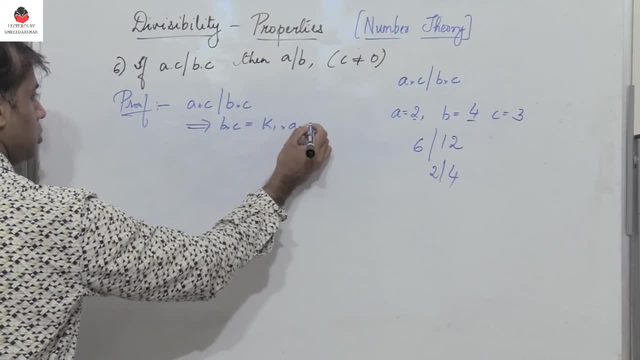 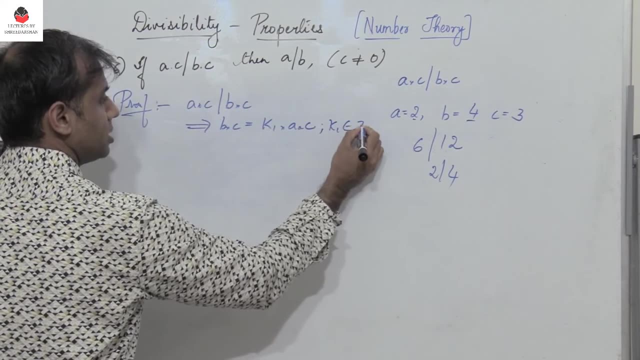 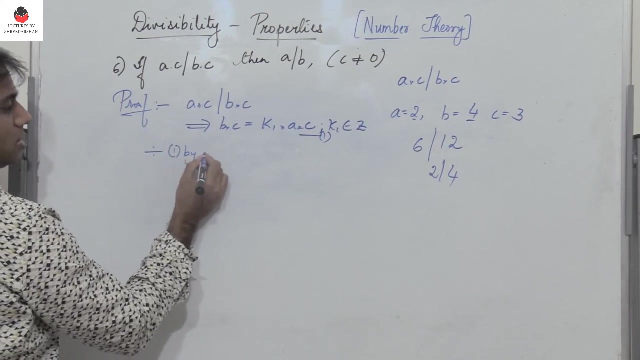 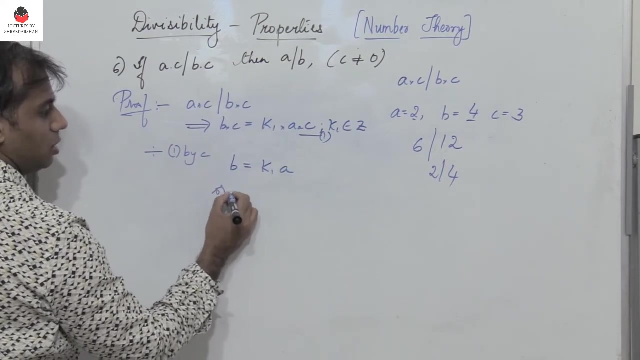 is equal to k1 into a into c. So b into c is equal to k1. into a into c, where k1 belongs to a set of integers. Call this as equation 1.. Divide equation 1 by c. So if I divide the entire equation by c, I get b equals k1 into a or a divides b. So very simple. 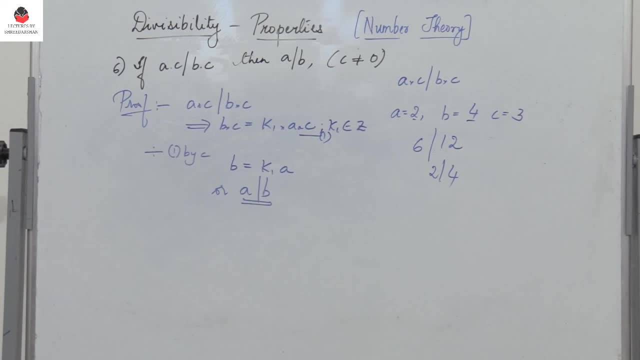 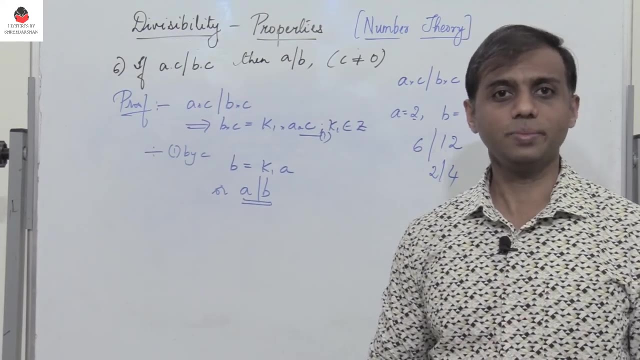 proof for this property. So this completes most of the properties of divisibility. So all the properties are very simple and we have- we have seen- the proof of all these properties by taking examples also. So do not forget to like, share and subscribe, and press the bell icon to get. 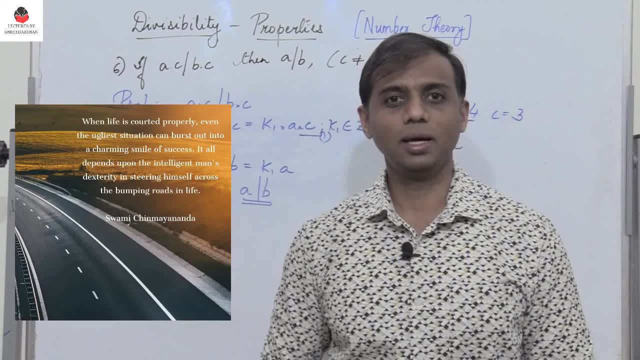 notifications of all the further uploads and click on the bell icon to view all the other videos in cryptography, as well as in engineering, mathematics, and thanks for watching.